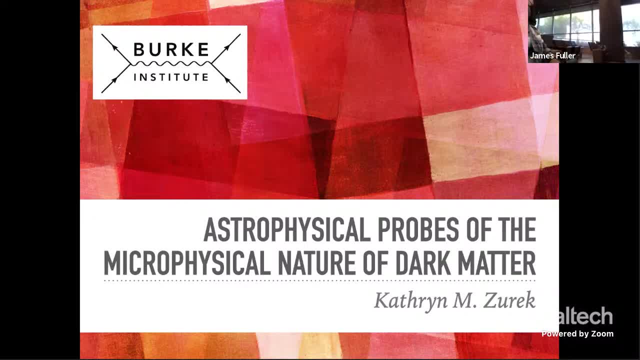 Yeah, of course, I think a lot. Okay, why don't we get started? It's great to see For those of you watching on TV. there's an almost full auditorium here, So you're missing out, And obviously everyone is very interested in this. 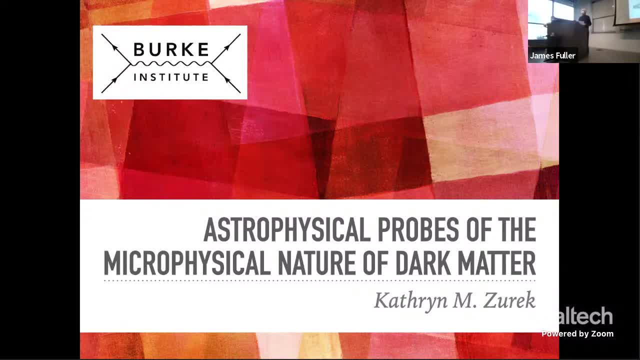 Our next speakers talk, so I. it's my great pleasure to introduce one of our own professor, Catherine Zurich, who joined the faculty at Caltech in 2019, right before the pandemic, And so I actually haven't met her yet in person, so 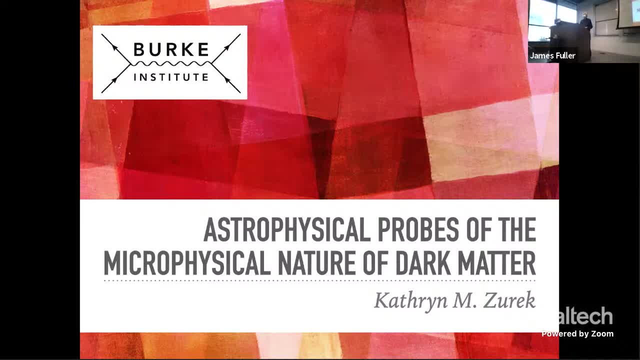 But she, like many excellent scientists, was, comes from the Midwest And was went to a small college in Minnesota and then the University of Washington in Seattle, PhD in 2006.. Then she has several distinguished positions: postdoc, SRAM fellow. 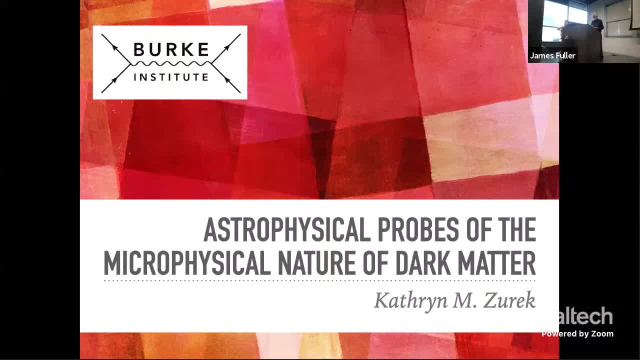 at a variety of places. she became an assistant professor at University of Michigan in 2009.. Associate Professor at in 2013.. She then went to Berkeley, and particularly the Lawrence Berkeley National Lab, And then she also was a fellow, elected a fellow of the American Physical Society, in 2017, and joined us, as I said before, in 2019, where she is pursuing. 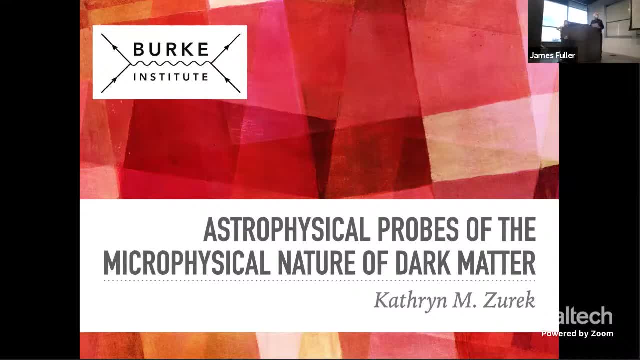 Previously a very interesting career studying new, new models of dark matter and how they may be tested by astrophysical observations as well as tabletop experiments, And recently she was- last year- named Simon's investigator, which is a very high honor as well, so it's a great pleasure that I give you Professor Catherine Zurich. 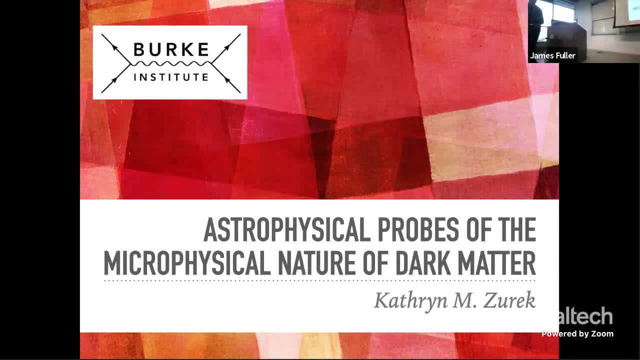 Okay, So thanks so much for the introduction and the invitation to give this talk. I'm excited to be here. I had originally been scheduled to come give this talk in Well, the spring of last year, So here we are. So I wanted to bridge really a broad range of topics. 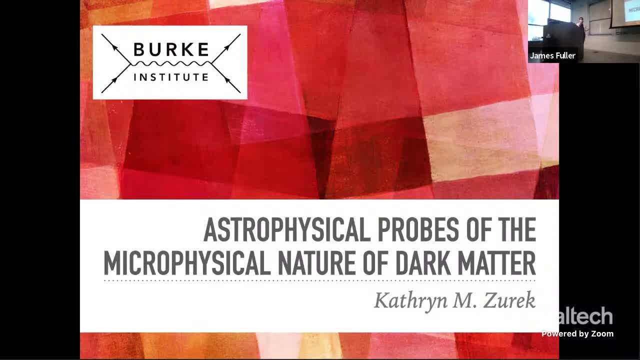 Because I want to throw a bunch of ideas And directions that I'm thinking about or have thought about as hooks for further discussion. and I'm really doing this this way because it's my home institution And I would love to start a conversation with all of you about things that I'm working on. 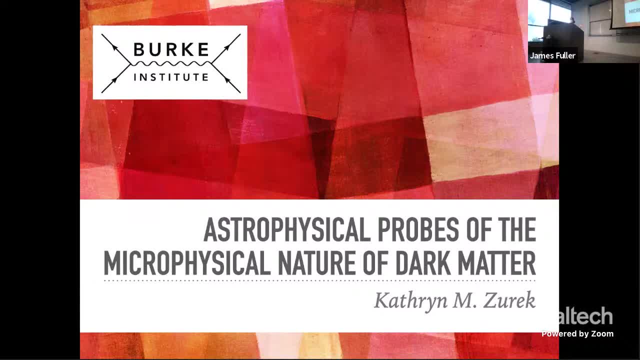 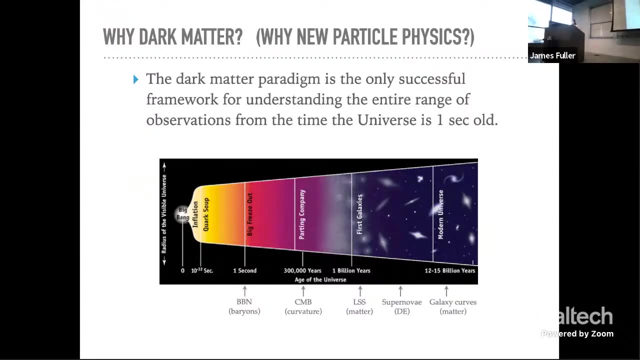 So it's. I'm attempting here to be broad range broadband without being scattershot, So so, let's, let's go down this path. so it's good to always. I enjoy starting this talk Just to remind ourselves, since we're standing in front of such a big problem, of how far we've come in understanding the evolution of the universe. 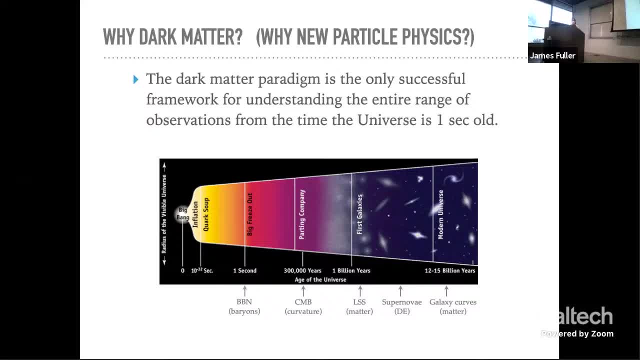 And the fact that we really need new physics beyond the standard model to understand the broad range of cosmological observations. So this comes from the time that the universe is a second old, down to the measurements of the cosmic microwave background epoch And the realize that there is a huge amount of time and we're still somewhere around the end of the year where the universe comes in. 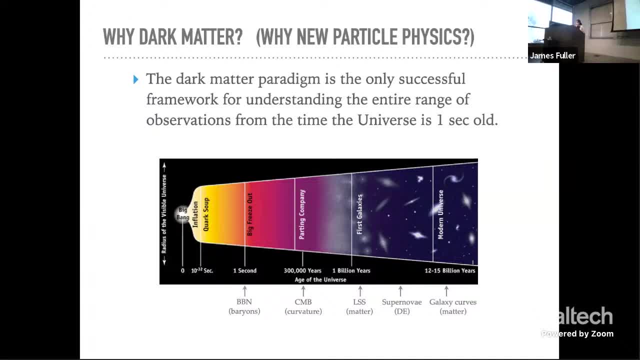 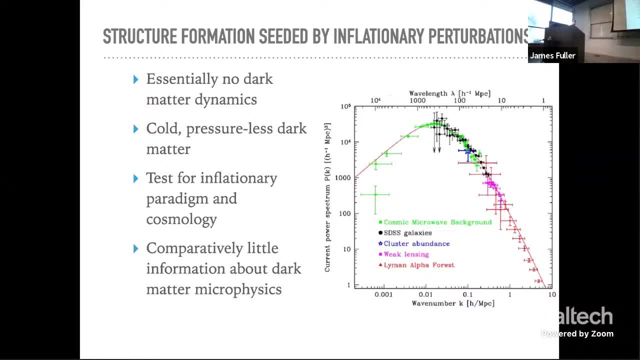 Where we will come to. But what I would really like to talk about is the whole idea that we are all connected to this world and we will happen to be connected to this world. And then how do we connect to the world from the star, to the moon and from the planet? and then how do we connect to the universe? 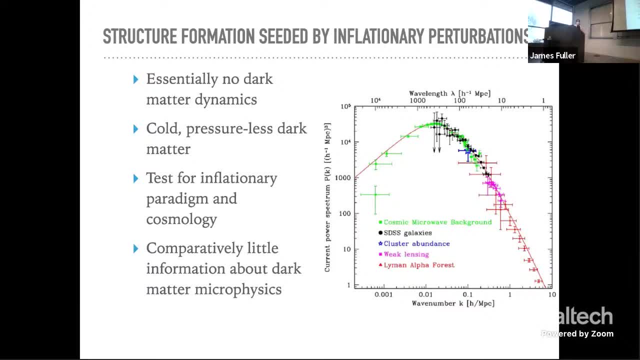 So the first pilot will be a light dark matter paradigm And the next one will be a dark matter paradigm, And this is non-relativistic, It's pressureless, which means that it just dilutes with the volume of the universe as it expands. So really, what we know in some sense about the dark matter is first and 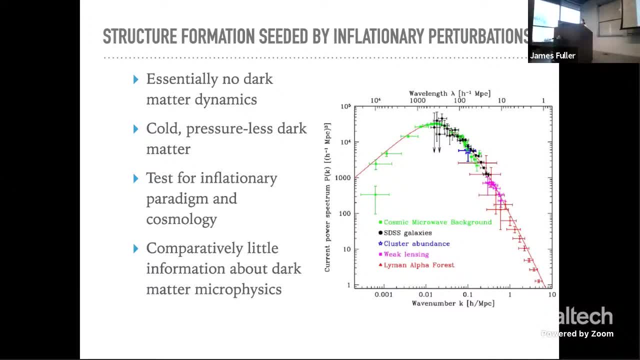 foremost, a test of the inflationary paradigm And the fact that we can measure this matter power spectrum. now, this plot is so old and so classic. I didn't even include a reference to the authors, but really what this tells us is that dark matter inflation seeds the scale and 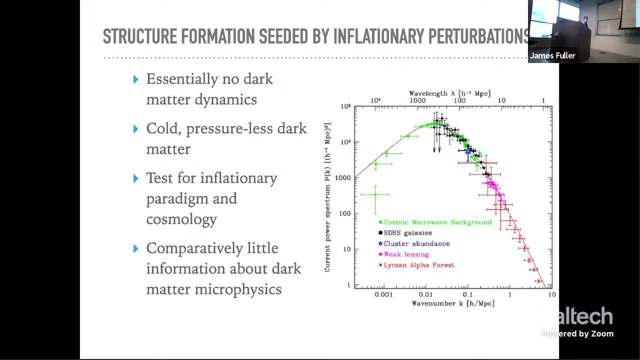 variant density, perturbations that just grow under the power of gravity and that allow all of the structure in the universe to form. as we see it, There is comparatively little information about the details of dark matter, microphysics. Now, the fact, the abundance, how much we can weigh, the 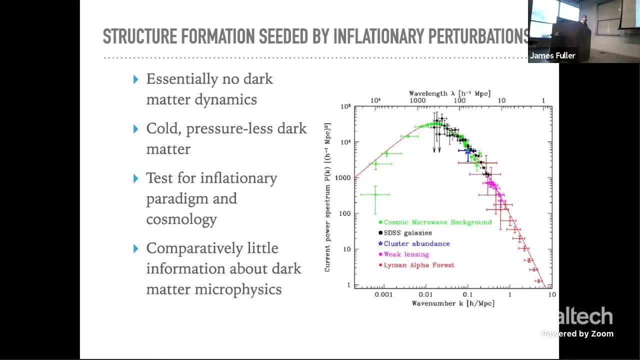 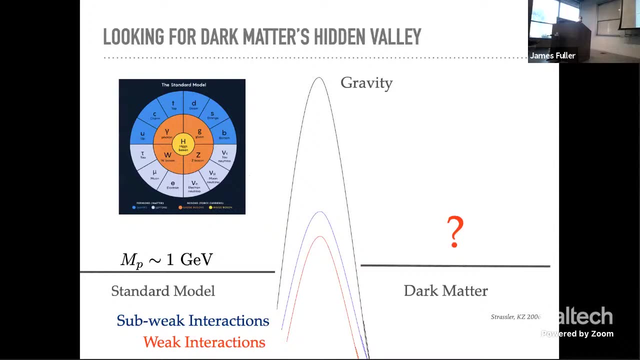 universe. so we know how much dark matter there is, We know that it has to be cold, We have limits on how much it can self-interact, both with us and with the dark sector itself. But so far we can't reconstruct the theory of dark matter the way we would like to be able to. 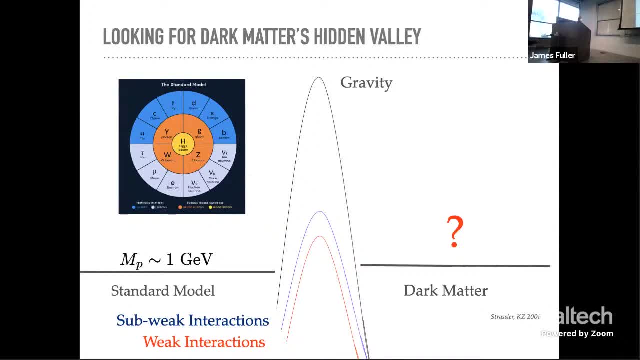 with the standard model. So we have this picture where the standard model has a very detailed theory associated with it. It has all this dynamics, the matter and the theory, And so we can't reconstruct the theory of dark matter the way we would like to. 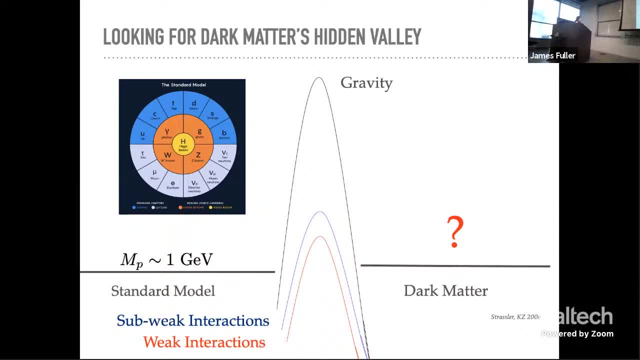 with the standard model. So we have this picture where the standard model has a very detailed theory associated with it, And so we can't reconstruct the theory of dark matter the way we would, and the gauge interactions. finally, the Higgs Boson: We know the mass scale. So if I think 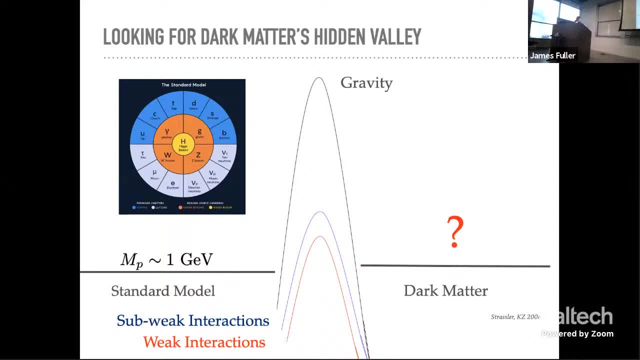 about. the y-axis: here is a mass scale and the x-axis here is something like an accessibility. So the standard model sets some mass scale. at the bottom of it you have the proton mass. The bottom of the baryonic sector you have the proton mass And then there's some barrier. 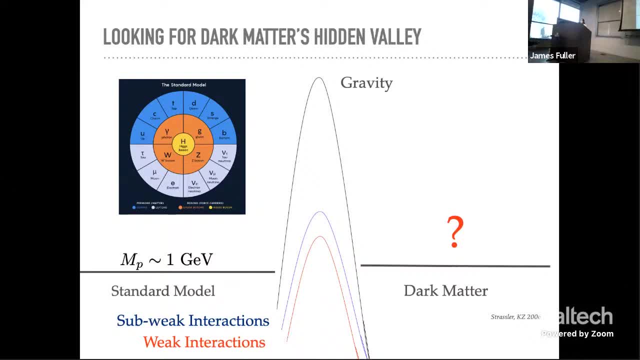 that separates us from the dark matter sector. We actually don't know how high that barrier is. We know, at minimum and half the along time, that this��eda is very changeable. according to Hossey's, to communicate with us through gravity, which is the weakest force, and all the information that we 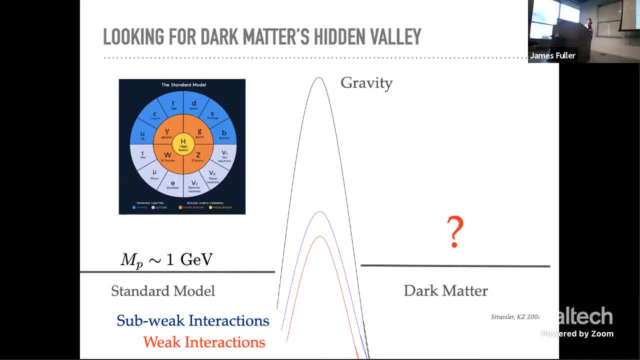 have about the dark matter comes only via this very, very weak force, and so, if you think about it, it's quite remarkable that we've been able to weigh it, we've been able to learn, you know, at least on large scales, how it's it: it collapses, okay. we, we know that. it's pretty well approximated. 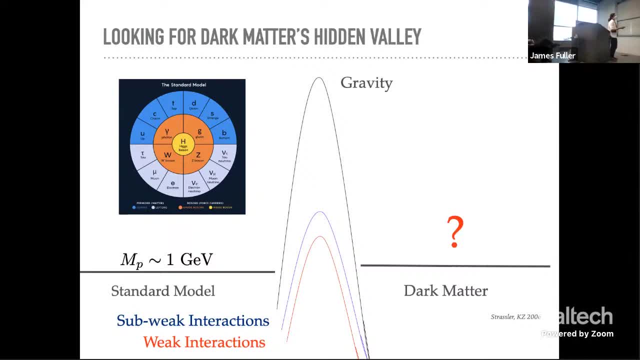 to be cold. we know that self-interactions can't be too strong, but other than that it's kind of a question mark. now we have assumed that it's very simple, but there could in fact be dynamics in there and we don't even actually know what this mass gap or this mass scale associated with. 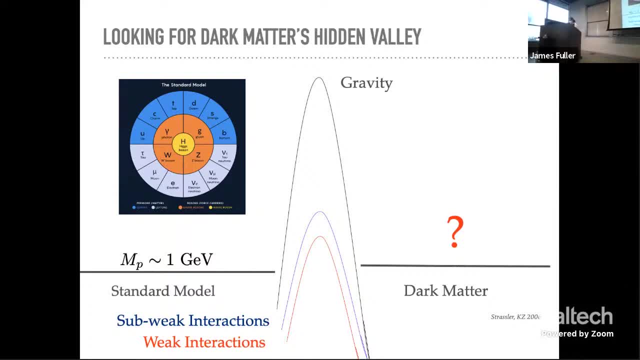 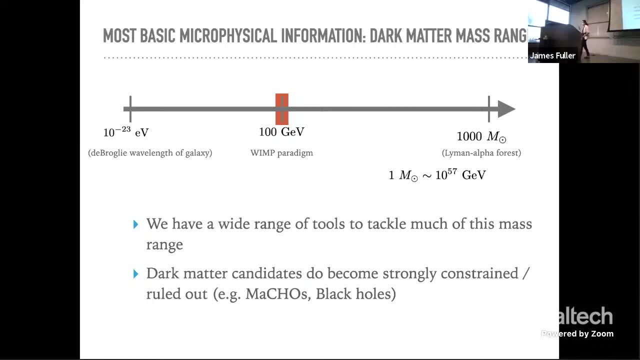 whatever dynamics is sitting in the hidden sector is okay. so particle physicists, at least traditionally, if we look back 30, 40 years, kind of collapsed this discussion onto looking at dark matter near the weak scale and uh, in fact, if you just look at what's astrophysically allowed, the mass range that's. 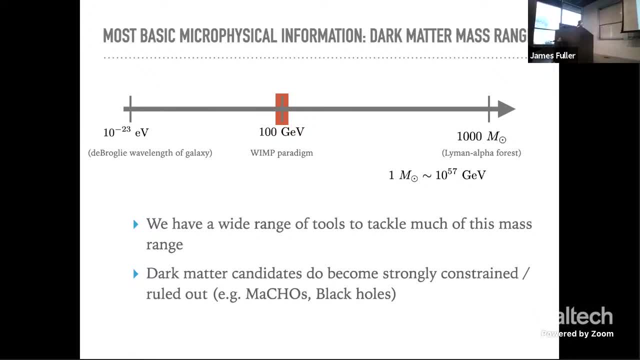 covered is from something like 10 to the minus 22 electron volts, or 10 to the minus 23- there's some uncertainty on that- all the way up to a thousand solar mass. so if you're a particle physicist who thinks about particle astrophysics, you know that a solar mass is about 10 to the 57. 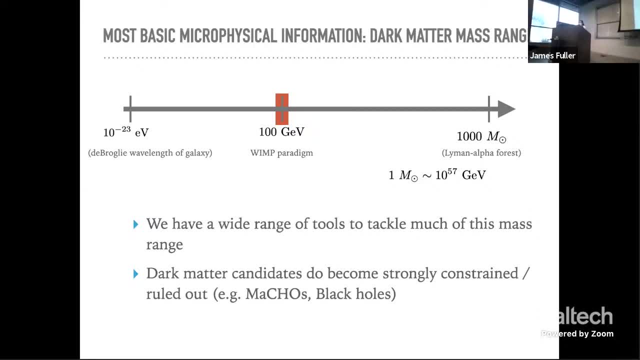 gb. okay, so you can count all the orders of magnitude that's allowed in that mass range. most of the searches of dark matter up until about five to ten years ago focused on this narrow mass window around about 100 gev. there were also, uh sort um astrophysical candidates for dark matter. 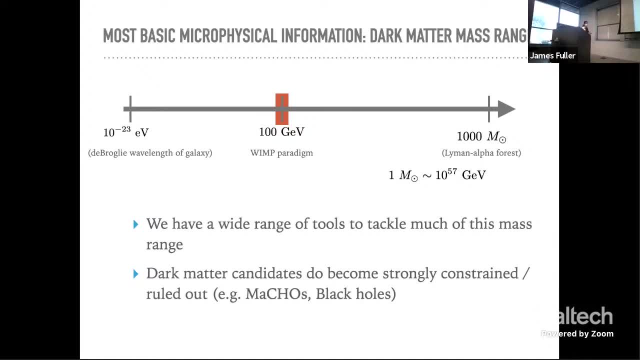 massive compact halo objects and black holes that have been mostly strongly constrained or ruled out. and so just to make a connection there, because this is really where a lot of the focus in the early days of the dark matter was on the dark matter and the dark matter was on the dark matter. 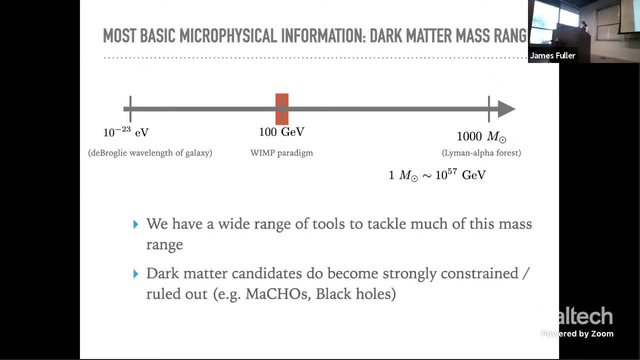 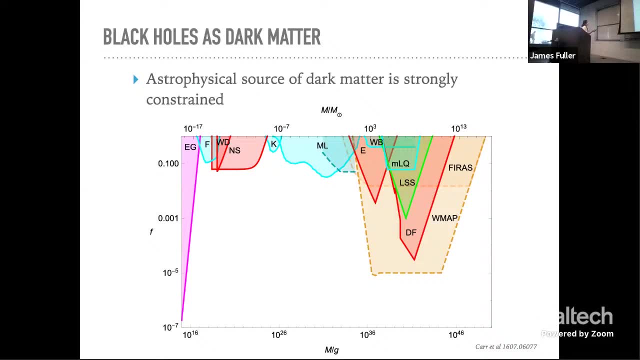 searches was on some type of astrophysical explanation and that's been pretty well covered. so, um, at very low mass, below about 10 to the minus 15 solar mass- black holes would evaporate. on the high end you would be able to see them through the, the graininess and the power spectrum. 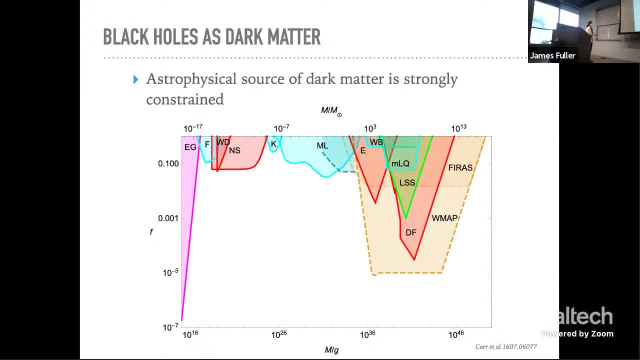 through the lyman elka forest. so there's a lot of different ways that that's constrained and over much of the rest of the mass range there's a whole bunch of different searches that constrain black holes as the dark matter. so on the y-axis here this is the fraction of the dark matter that can be in. 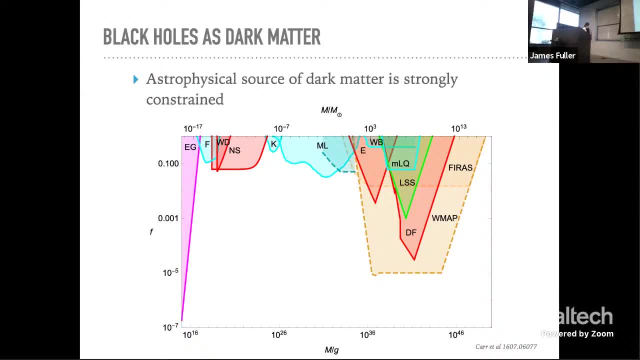 such an object. now this is still an ongoing area of research and you hear people talk about shifting these. you know especially where there seems like there might be a little window about whether you can lift those constraints just by the astrophysical uncertainties. but more or less this is the 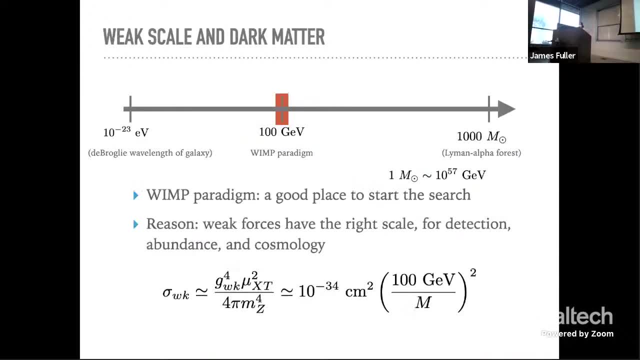 picture, and so what we're focusing on is physics beyond the standard model and, as i said earlier, what we're focusing on is the weak scale, and i don't want to denigrate this focus because i think it's a really good place to start, and the basic reason is that the weak forces. well, first of all, 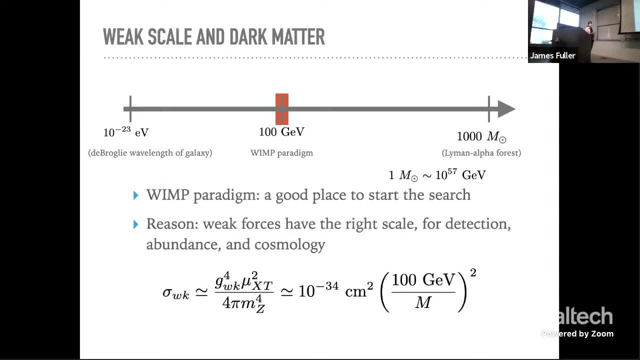 they're known and they have the right scale for detection, which is important for learning something about the microphysical nature, for the abundance and for the cosmology. so just to do a little bit of naive dimensional analysis here to kind of set the scales that are going to recur. 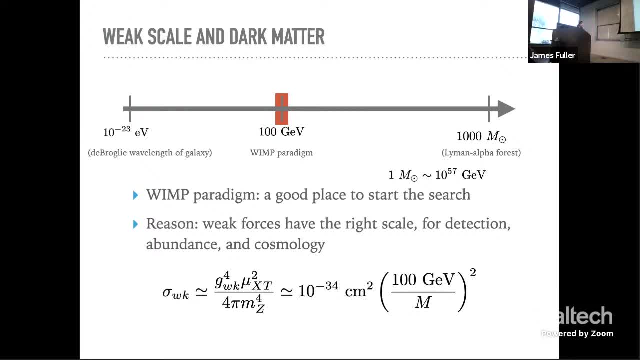 several times throughout this discussion. this interaction- a typical weak interaction cross section- has a weak coupling constant. it has a reduced mass between the dark matter particle, which is always going to be x, and whatever the target is okay. so oftentimes this is a nucleon or a nucleus in a direct detection experiment and then it's mediated by the weak force around 100. 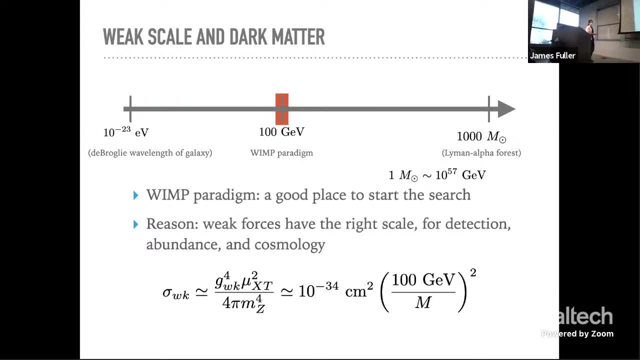 gev. so that comes out to be about 10 to the minus 34 centimeters squared. it's actually smaller than that because this reduced mass brings the cross section down more into the 10 to the minus 38 centimeters scale. so i said that this weak kind of cross section is about right for setting the. 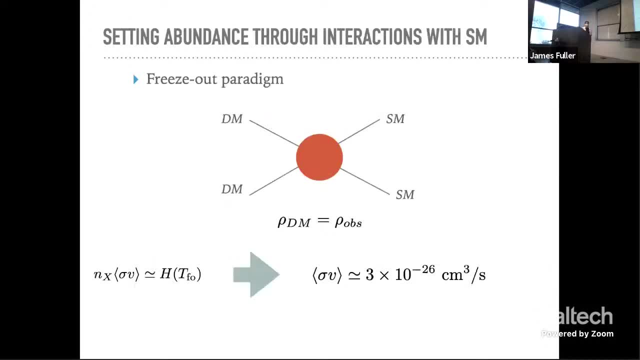 abundance. so that back of the envelope is also pretty easy to do, because the process that sets the macroscopic come on a dark matter that we see in the universe happens through a microscopic process. it's dark matter, annihilating to produce some pair of standard model particles. 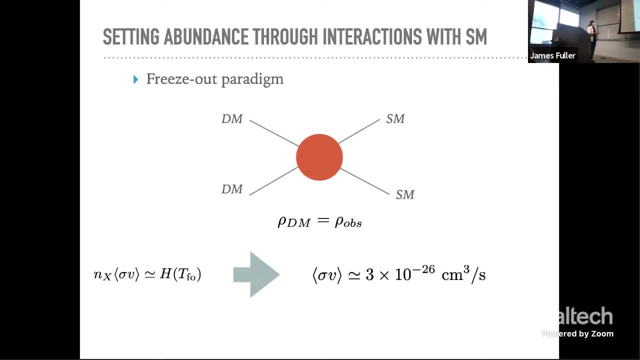 through some interaction which is mediated by the weak force, and so you can compute the amount of dark matter so they annihilate, until you have so few of them that they can't find each other to annihilate anymore. this is the standard freeze out calculation, so you compute the rate of the 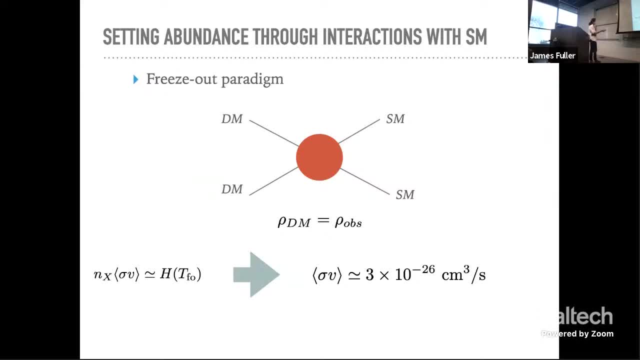 annihilation. it goes like the number density times this microscopic interaction cross section. and then you set it equal to the hubble expansion when they can no longer find each other, and this because you measure the amount of dark matter in the universe. that's an annihilation cross. 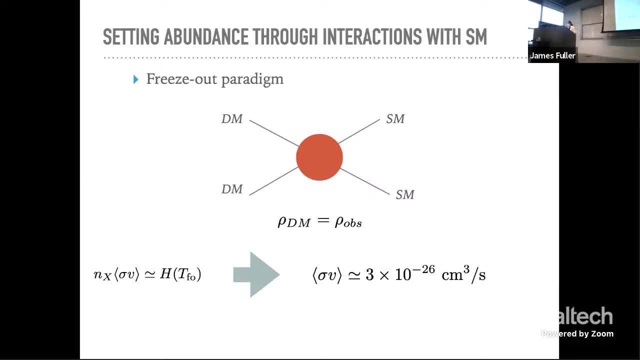 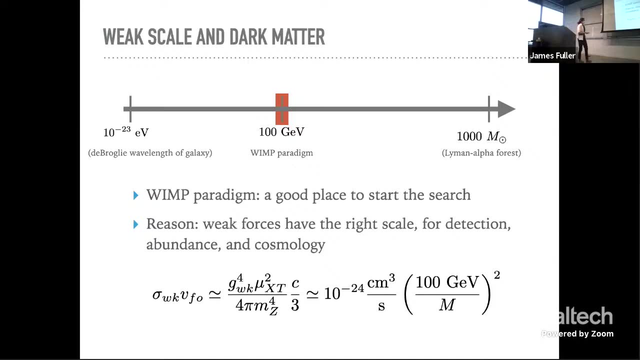 section which you might want to remember, is about 10 to the minus 26 centimeter cube per second. so now you go back to that back of the envelope that i just presented on the previous page. you take that cross section, you multiply it by seed of light, because they're just starting to. 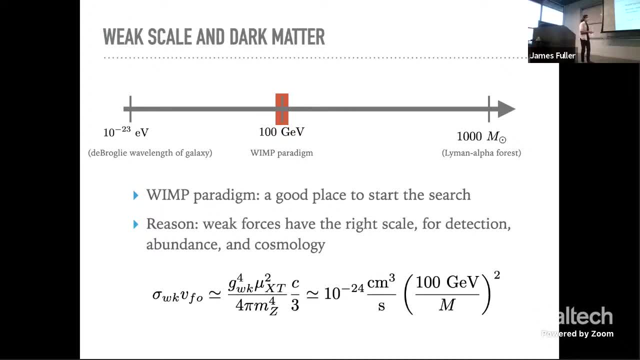 become non-relativistic when they freeze out- and the answer is about 10 to the minus 24 centimeter cube per second for 100 dv dark matter. so when you talk about dark matter being at the weak scale, but we really mean it's about dark. 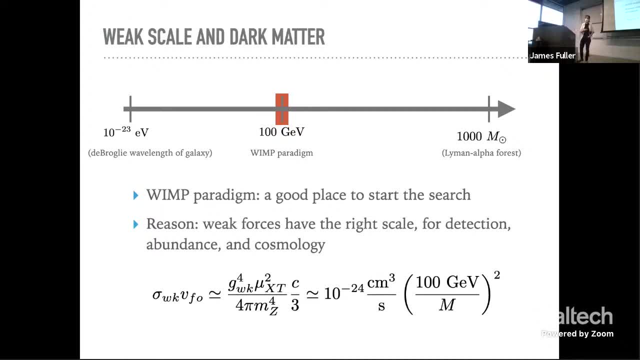 matter, that's a couple of tev, turns out to be the right number. okay, and this is, i think, very powerful motivation to look for dark matter with mass around a couple of tev and um, this, in fact, is what the lhc program is aiming for- actually does not have an amazing direct sensitivity to. 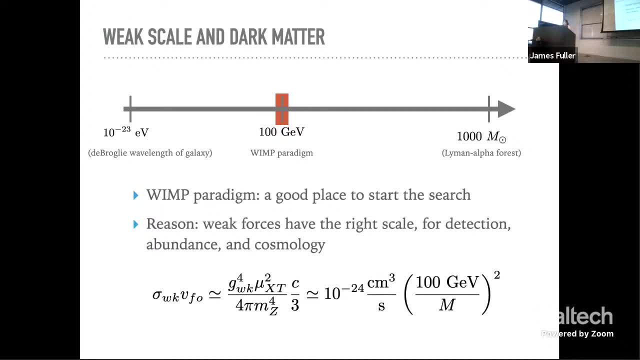 weak dark matter, which would be the subject of another talk. it's the um, the target of direct detection experiments looking for dark matter at the weak scale, which we'll talk briefly about later on. but we're going. you know we're still looking for this candidate and it's still viable now. 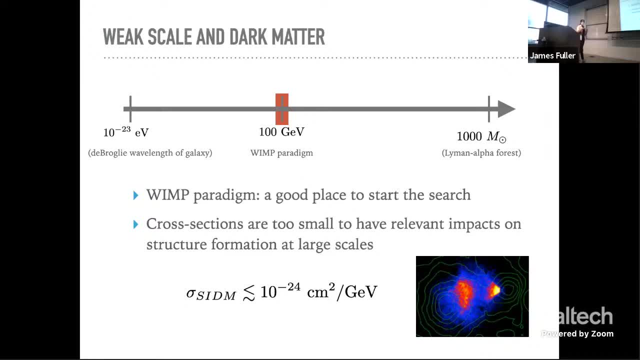 it has astrophysical impacts that have, uh, deeply formed the way that we look for dark matter in astrophysics, and it's the fact that i alluded to earlier, which is that dark matter is the target of dark matter in the wimp paradigm, because it annihilates, it freezes out, it has. 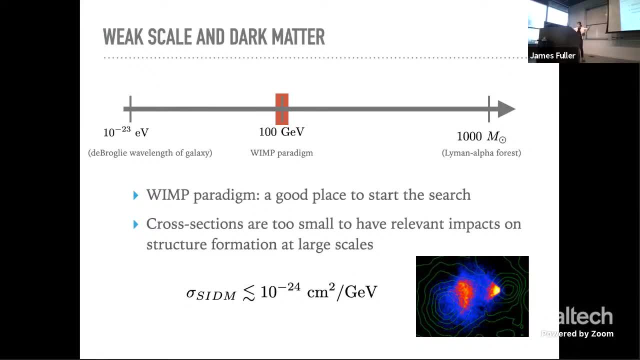 its relic abundance. it expands with the. as the universe expands, you know it dilutes and that's about all it does. you might be able to see it through its annihilation. maybe if you look towards the center of the galaxy, there are pro. there are searches ongoing for that, but in general, 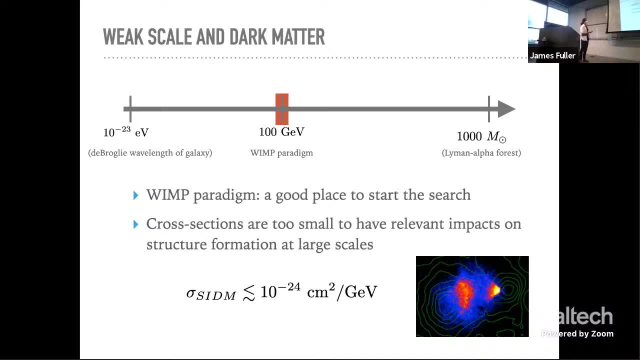 in order to have some uh impact on structure formation at large scale- and when i say large scales i mean galactic scales are larger- the interaction cross-section actually needs to be bigger, much bigger: 10 to the minus 24 centimeters squared per gev. so you recall earlier i said weak interaction cross sections are not really bigger than 10 to. 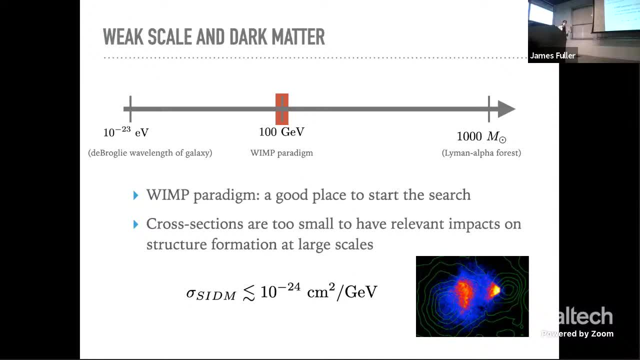 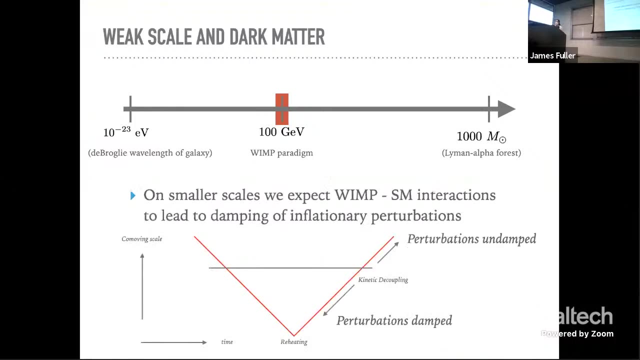 the minus 34, and so this is really just way too big. so so, in terms of what we see in the universe, it's just not relevant for the formation of structure, and so gravity really does all the work for us. however, this is on large scales. on smaller scales, this isn't really true. in fact, it's not true. 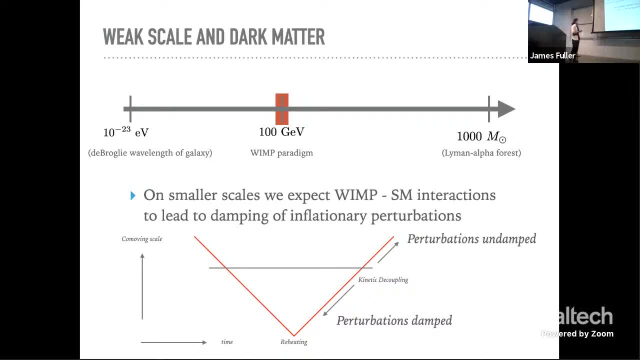 on smaller scales. we expect dark matter center model interactions to lead to the damping of inflationary perturbations. okay, so the way to think about that is dark matter. in the early universe, the temperature is high. weak interactions are not weak at high temperatures, so there's rapid 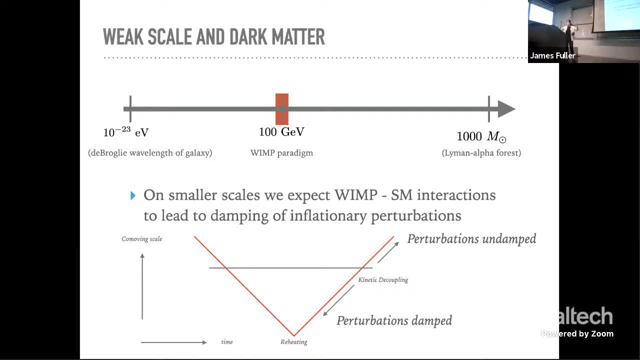 scattering between the dark matter and the baryons and that proceeds until the universe drops to a low enough temperature that that scattering, not just the annihilation but the scattering process decouples. and so as long as there's that strong scattering process that's going to erase the inflationary bun, the inflationary perturbations. so if you look at the 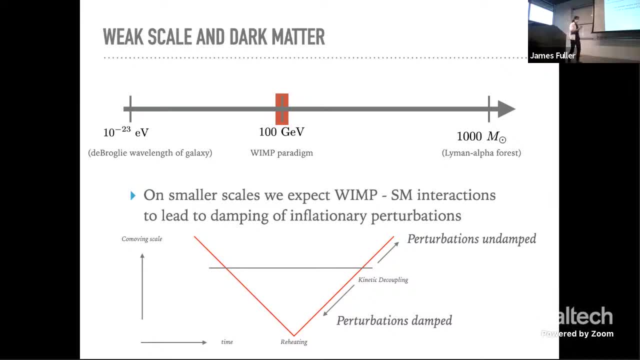 co-moving scale as a function of time. there's this cosmological goodbye and hello again effect, to quote colvin turner, where a perturbation of a given scale leaves a horizon and then eventually, after reheating, it enters again, and so the question is whether that perturbation is inside or outside the horizon when kinetic decoupling occurs. okay, if it's inside. 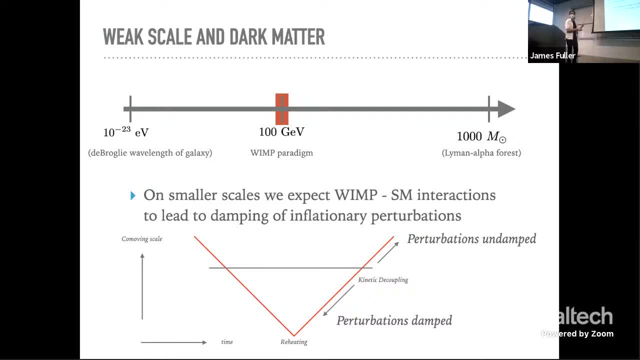 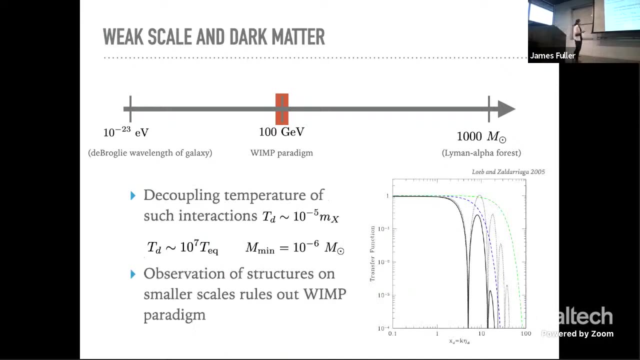 the perturbations are gone, i'm not going to have any structure at all. if it's under, if it's uh, if it's outside, then i'm going to just have the ordinary inflationary story go on uninterrupted. so you think, calculate this and the decoupling temperature is actually very low. it's um, you know it's above. 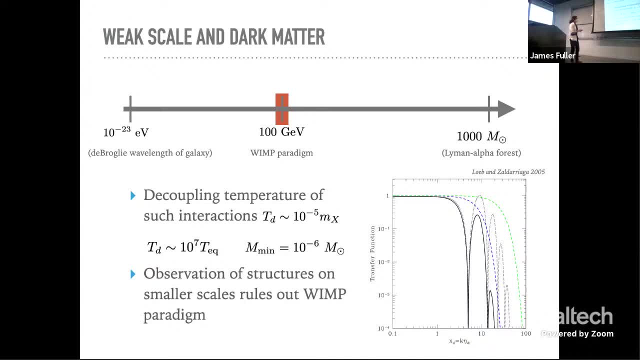 an meb, but not by very much, and so that corresponds to a minimum halo mass of about 10 to the minus six solar mass. so when you hear people talk about in simulations testing the minimum halo mass, that is not a test of the cdm paradigm, that is a test. 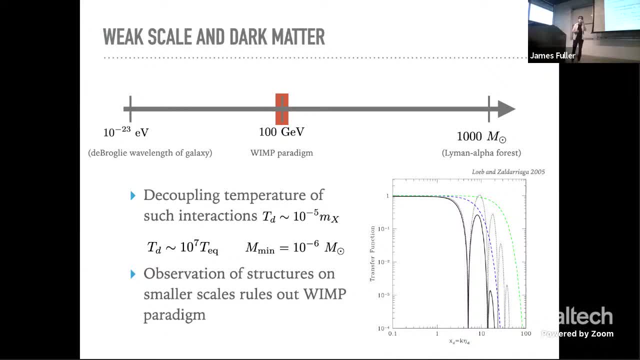 of the wimp paradigm and it is. it is particular to the interactions of that, that paradigm. okay, it is not true in general. in general, i can have some hidden sector. it can be the case that dark matter doesn't reside here at the weak scale. it's perfectly viable to say, be at a lighter mass scale. 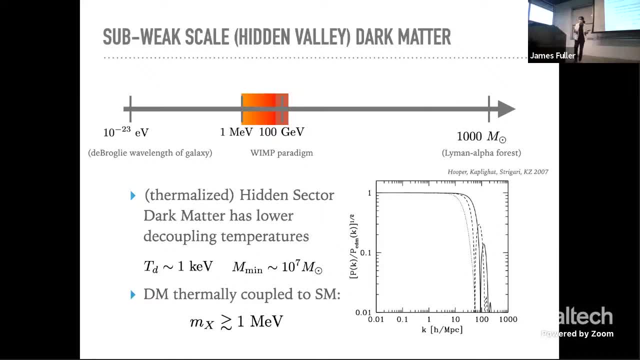 it's at a lighter mass scale, the forces that mediate the scattering tend to decouple later, so, as a result, the typical mass scales where you're going to erase those perturbations are larger, and so you can easily have a situation where this minimum mass could go all the way up to about what would be allowed. 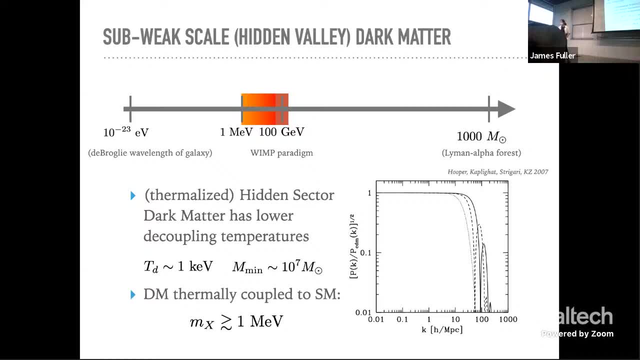 with the lyman alpha forest, which is on the orders of something like 10 to the seventh solar mass, and typically what that corresponds to in terms of dark matter mass is: you push this mass down from. you know, uh tev scale down to an nev. so that's about six orders of magnitude in 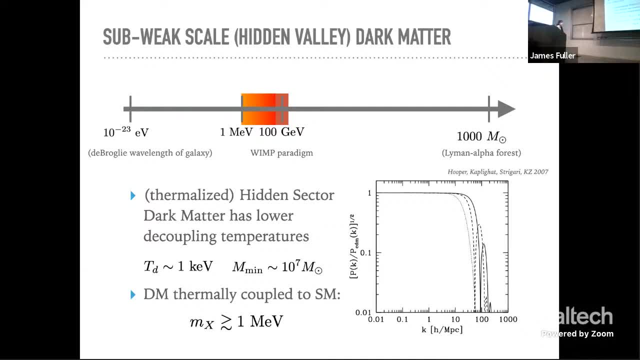 mass. it's quite substantial and in fact you would be able to see now this damping of perturbations on much, much larger scales if you were able to measure the dark matter power spectrum on those scales, which we can't currently okay, but which we're going to talk about- how you might be able. 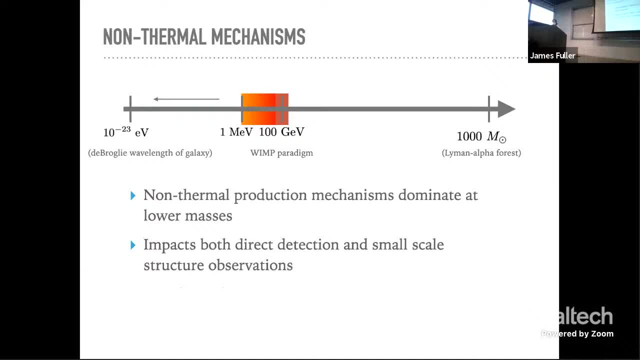 to do that. so, as i said, it impacts both direct detection and small scale structure observations should say that, as the date of the irregular OCLX dark matter mass drops below an MEB, typically the mechanism for setting its abundance is not through these thermal interactions that I've just been talking about where dark matter comes into. 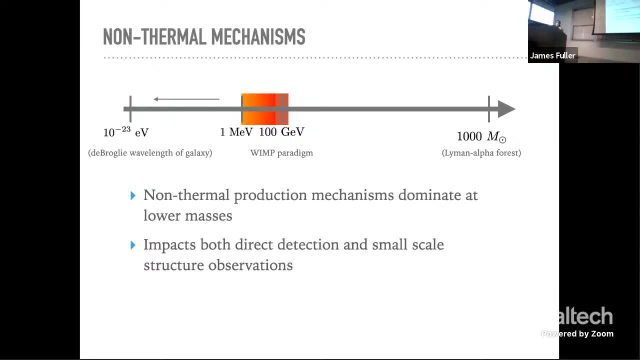 equilibrium with the standard model. It has to be populated in some ways, some different way. I'm going to talk about two right now that actually impact the way structure forms on small scales. So let me give you two kind of classic, relatively conservative examples. 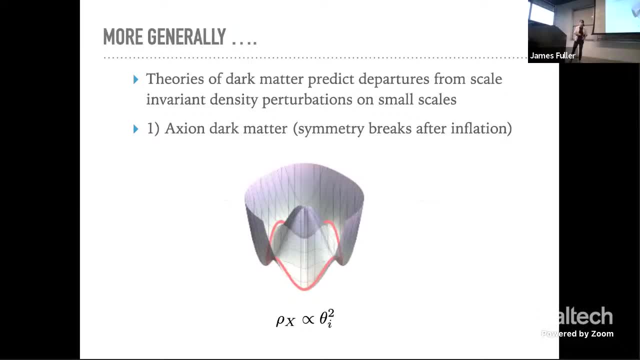 So axion dark matter. So axion dark matter originates from a complex scalar field with a structure of the potential which is not so different from the one that the Higgs boson has. Mass scales are completely different, but it has this wine bottle potential. 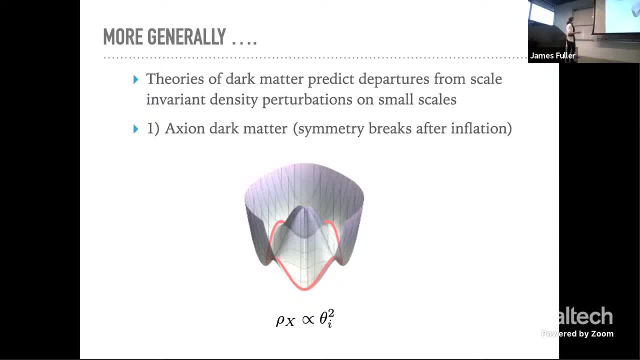 A difference with the Higgs boson is that in the angular direction there is an actual potential here, And so what happens is in the early universe. initially the field is up here at the unbroken part of the potential, And then as the universe, 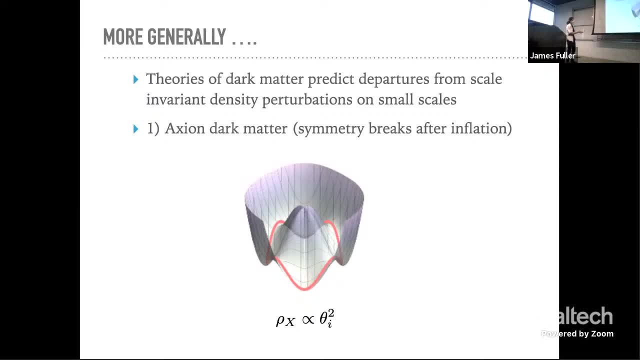 cools, it rolls down and it picks out some direction in this potential. And that potential is not flat. So depending on where it happens to land, the local dark matter density is going to be different And in particular it depends on what the angle is here. So once you actually produce, 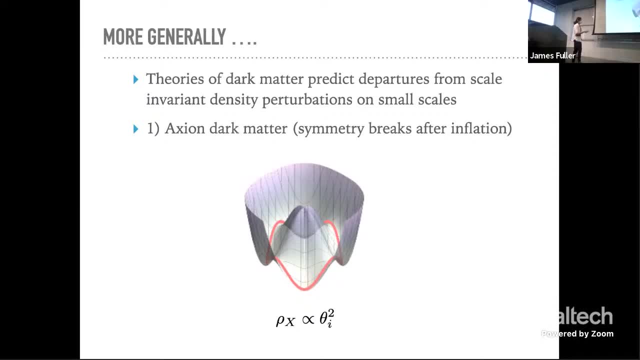 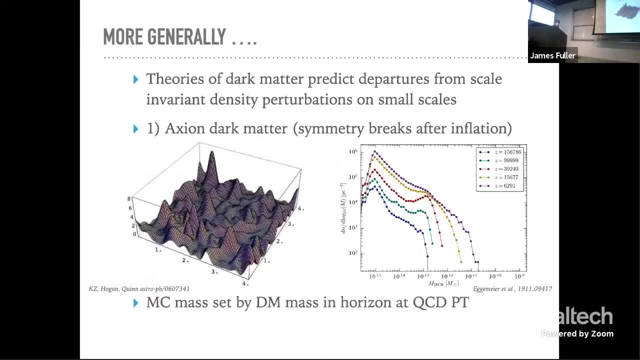 cold axion, dark matter by the oscillations of the field about the minimum of the potential. what you get on very small scales is huge density perturbations. So here, if you plot the density perturbations as a function of the cold moving, 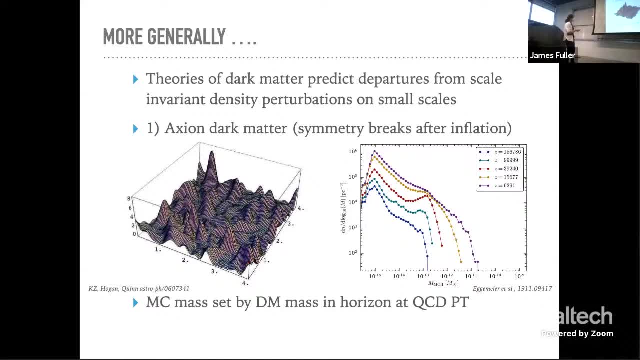 scale. so here's just a 2D slice. The only point I want you to take from this is that there are density fluctuations which are order one and in fact even larger, and that they're smooth on scales which are the horizon size at the QCD phase transition. 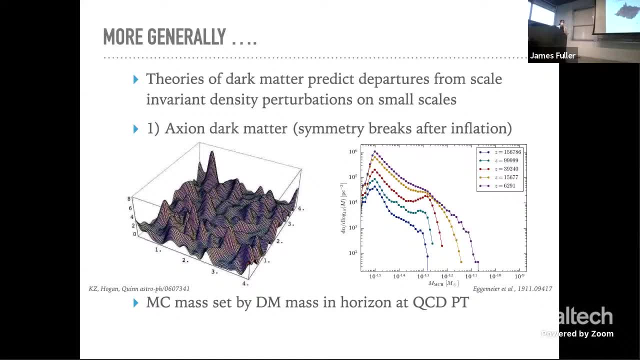 Which happens at temperatures around a GEV. So what you do is you look at the mass of dark matter that's within the horizon at the QCD phase transition and you compute it. It's a little more subtle than that, because the axion mass is actually just turning on as the QCD phase transition. 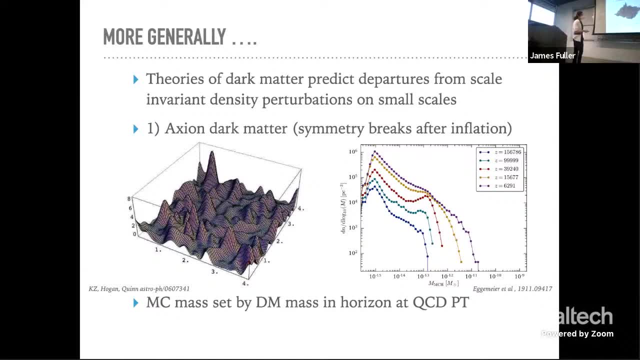 happens And that allows you to compute a halo mass function from the axion dark matter model. So that's what's plotted here. This is the halo mass function as a function of the mass And you can see that it's peaked actually down around 10 to the minus 15 solar mass. 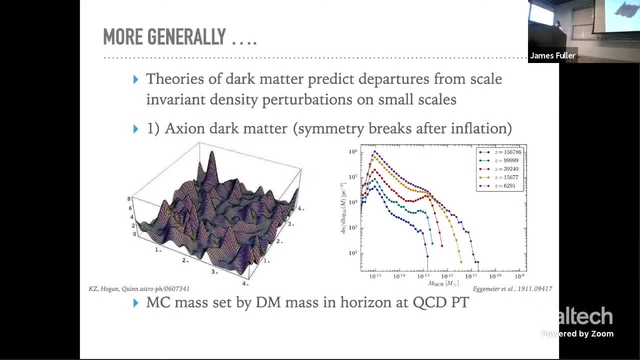 So here's one very classic, I would say, from a particle physics point of view, simple mechanism where you see very large amount of substructure, but on very, very small scales. In addition, because this overdensity starts out very large, the concentration parameters of these. 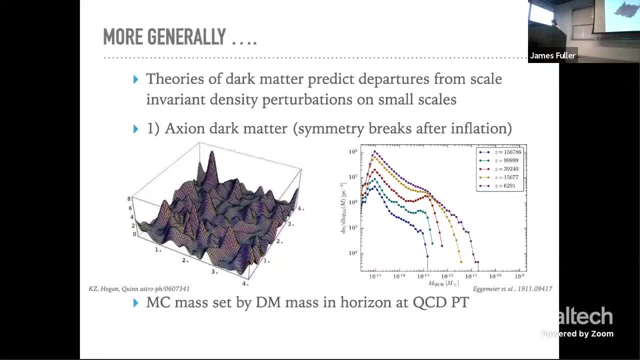 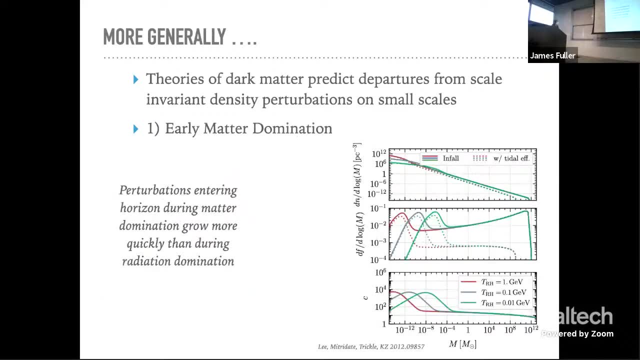 halos are very large- Okay, they're in excess of a thousand. These are much more dense and than ordinary CDM halos. A second example- should have changed this to two- is the case of early matter domination. So, quite generically, or in many models, I can have particles that are long-lived. 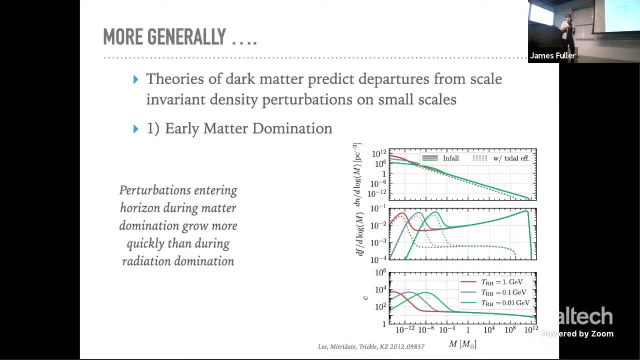 And when they're long-lived they don't. they become non-relativistic, They start to dominate the energy density in the universe and they cause matter domination to happen at temperatures way above the electrovolts scale, where they do in the standard CDM picture, And so what that does is 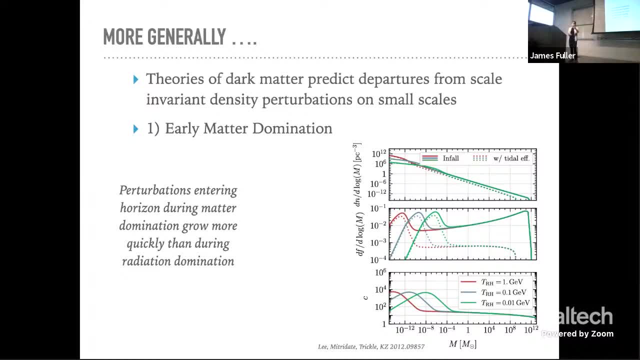 coming back to this picture, is any perturbation that enters the horizon when that early matter domination happens, now starts to grow linearly, just like it does late in the universe, And so you can get in on top of the ordinary CDM. So this is as a function of scale. This is a standard for 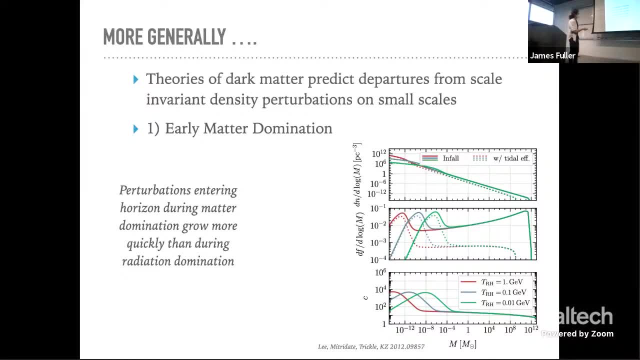 the halo. So this is the halo mass function. This is multiplied by F. But anyway you can get these additional contributions that depend on the temperature at which that heavy state decays. So this is a very another, very easy way to actually seed structures. again, very low mass. 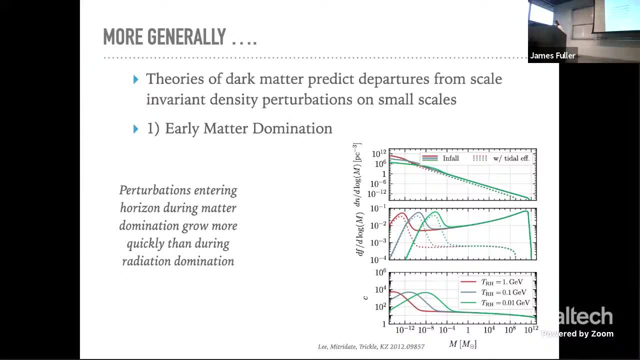 structures. So your next question is: well, this is a, this is a fingerprint of what's happening in the dark matter sector at very early times. Is there any way that I could possibly measure the matter-power spectrum of dark matter and get some idea of whether there? 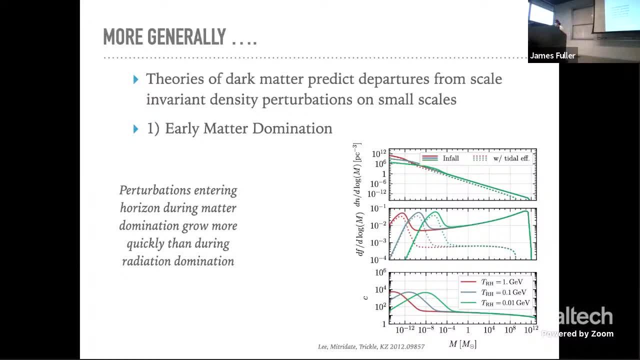 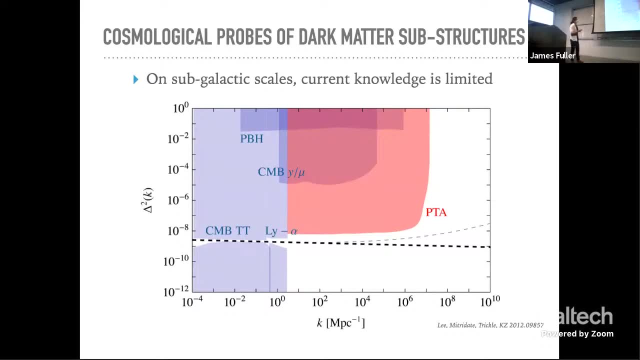 are substructures on those kinds of mass scales And the fact of the matter is that onute gallactic scales. our current knowledge of the matter-power spectrum- so these are the over densities- is actually quite limited. So you know, we have very precise measurements with the CMB. 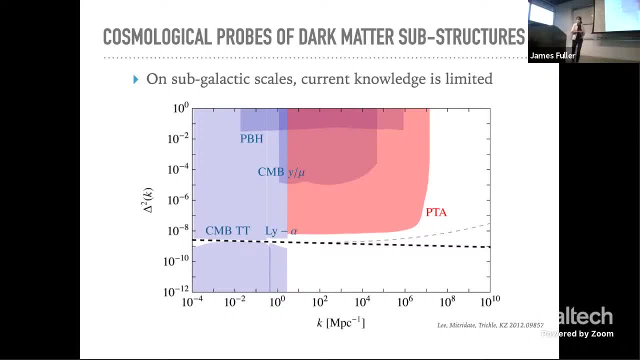 We have less precise measurements, but still reserved Jesus Crueba dealli. we have less precise measurements, but still still measurements with the Lyman alpha forest And then as you go to higher wave number, we just currently have little to no information, So I want to spend a little bit of time. 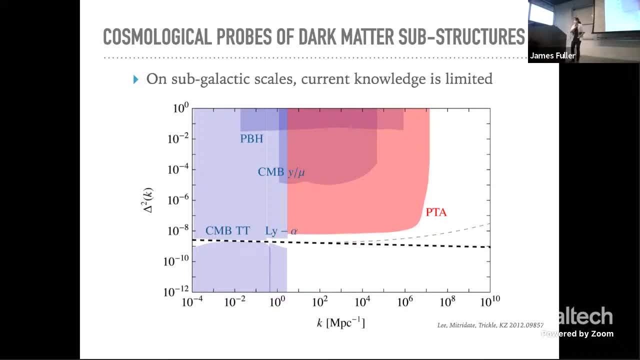 proposing some ideas. Now you know I'm not going to say that we're going to be able to go out and do these measurements like next year. These are long-term goals, but we need to spend more time thinking about how we probe the matter- power spectrum on these small scales. 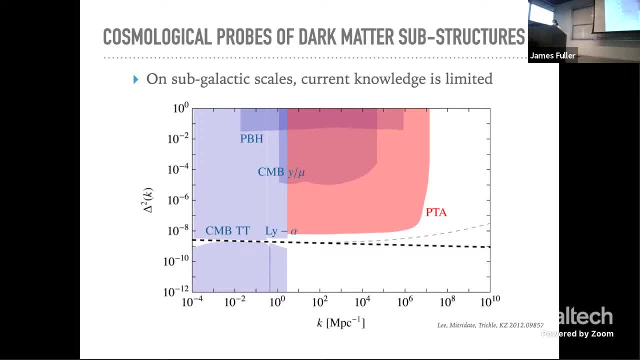 so that we can learn something about the microphysical nature of the dark matter. So I'm going to spend a little bit of time talking about PTAs, which is something I've been working on in the last few years. So here's a summary plot. 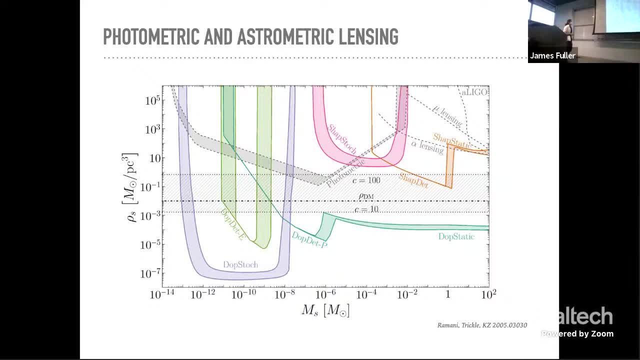 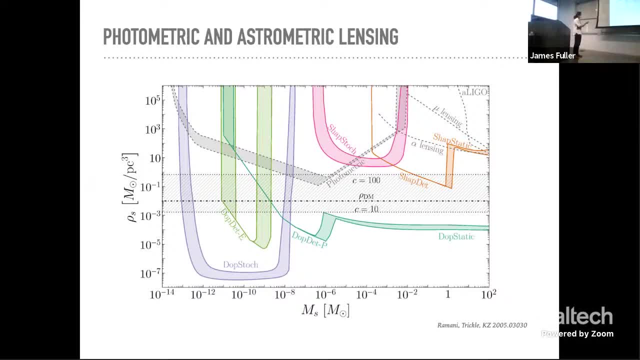 it's actually the density, but it's the standing, for the concentration parameter is a function of the mass of the handle, And so, just to orient At you, TDM has halos that have concentrations in the tense, And so you can see. now, here are different types of PTA searches. Okay, And what they? 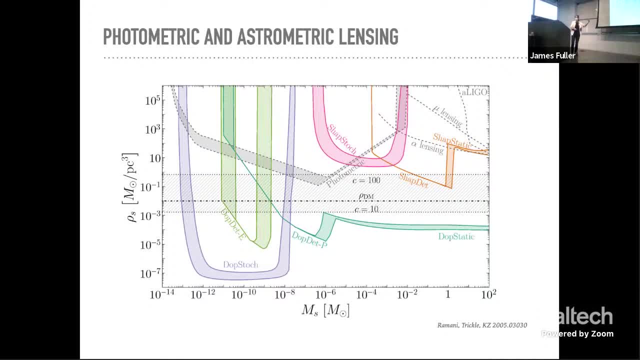 could do now. this is a futuristic Ska type measurement- which I'll talk about very shortly- where you're able to measure 100 plus pulsars over the timescale of decades. But you can see that in principle. now you can start to search for dark matter subhalos. 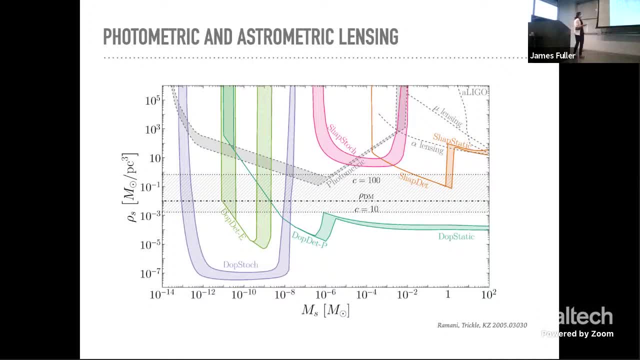 in that mass range. There have also been other proposals that I'm not gonna talk about. We put them on this plot due to other people and I encourage you to take a look at them if you're interested with photometric and astrometric surveys that in the future. 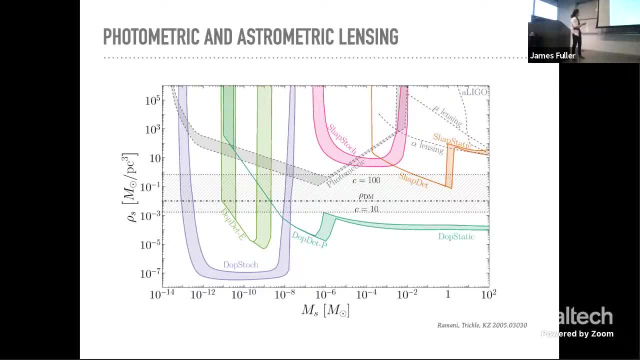 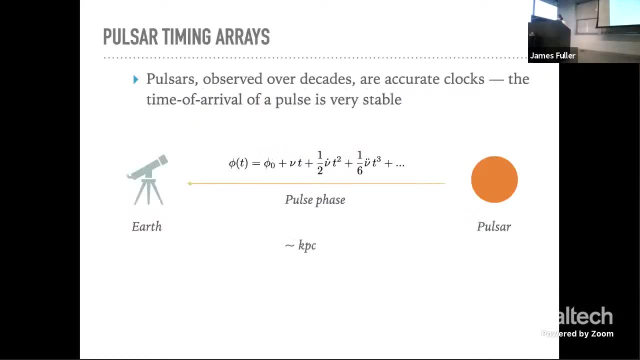 are not quite as sensitive in terms of low concentration halos, but can also reach a similar mass range. So what's the idea with pulsar timing arrays? So here's my cartoon That pulsars are really very stable clocks and that's what we're interested in using them for. 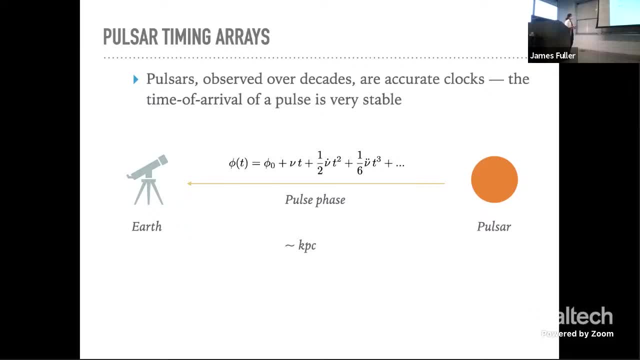 that they pulsars emit these pulses. they arrive at the earth. we measure them. I shouldn't say I measure them, but pulsar timing. observationalists measure it And there's a pulse phase And the thing that's remarkable about it- 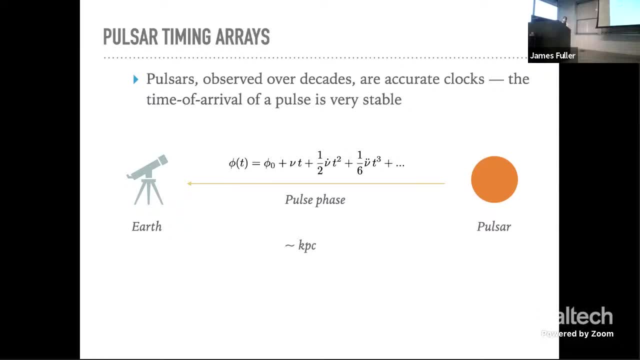 is that they fluctuate but they don't accumulate. okay, It's a good approximation that we can measure this pulsar over decades in some cases, and I can fit it with just some fixed number, the period, and with the first derivative of the period. 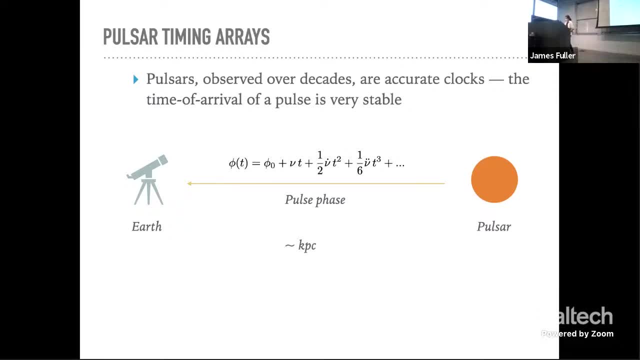 That's all that you need to actually predict the time of arrival of the pulse over the timescale of decades, the remarkably stable clocks. So the idea is that these pulsars, of course, are not in an empty environment. They're in the environment of dark matter, subhalos. 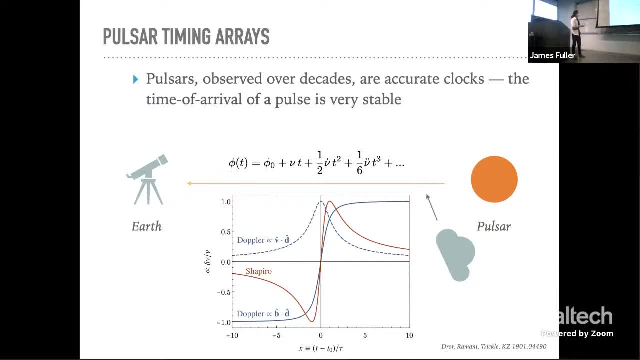 And really what happens is you can have a collection of these guys or a single one, and it can either pull on the pulsar or on the earth or it can give rise to Shapiro delay, And those have typical timescales associated with these processes. 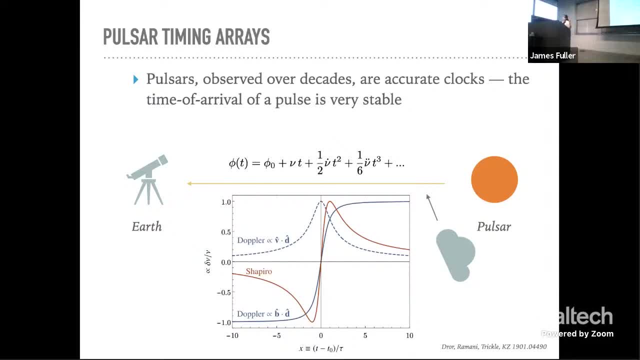 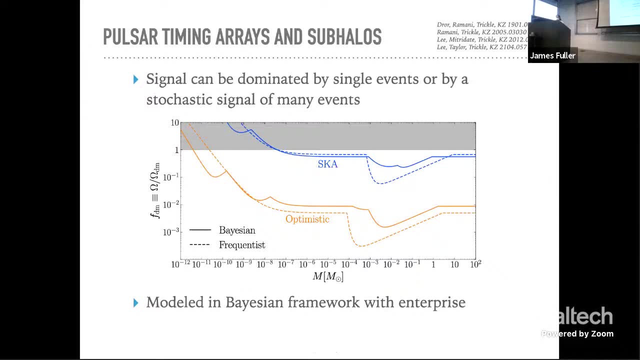 And the question is whether they have a large enough amplitude that you can see these above the noise that they already observe in their experiment. So we asked this question and we teamed up with at the end to get a more realistic picture- Steve Taylor. 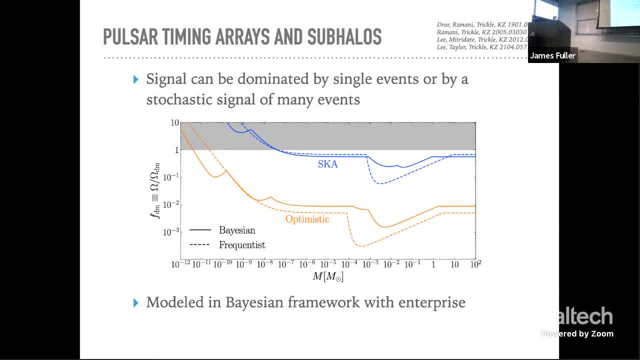 who also has some work on nanograph, to look at what you might be able to do in the future in terms of the fraction of the dark matter and a subhalo of mass m with an SKA type instrument or in some very optimistic far future type scenario. 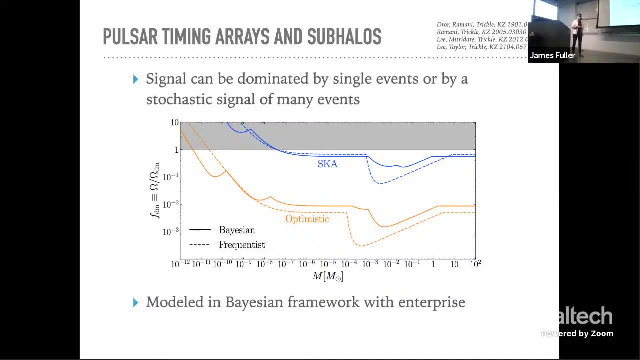 You can see that this is not granted. we have not taken into account, for example, a super massive black hole background. stochastic gravitational wave background will complicate this, But you can see that you have, at least at the theoretical level, sensitivity to dark matter. that's at the level of the density of dark matter that we observe. 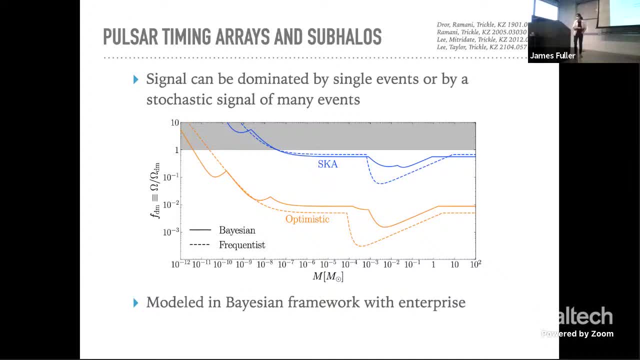 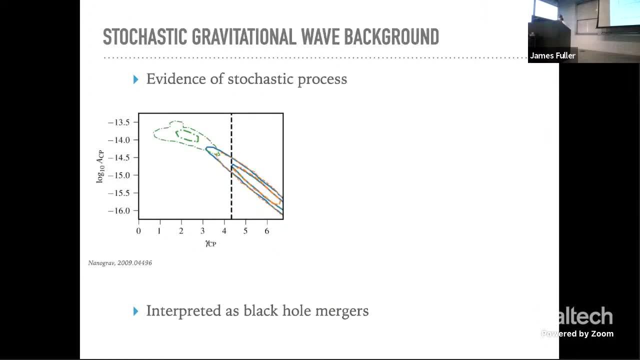 And that perhaps in the far future we may really be able to nail this down. Now, as I said, there is in Nanograv. there is evidence for a stochastic process in their data, which they have fit by a cosmological population of supermassive black holes that are emerging. 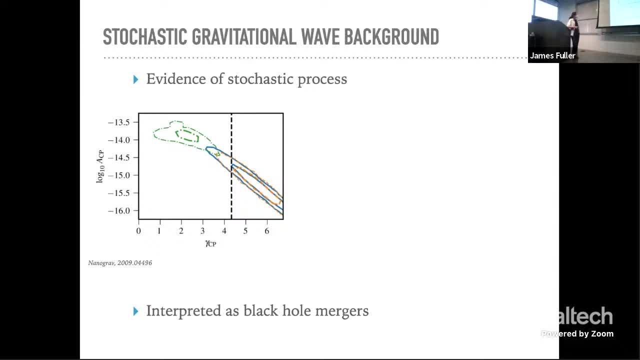 And the fit. you know this is the prediction of the model here and the amplitude, which is a little on the high side from what the theory would have predicted, but actually in quite good agreement, And so this fits well. it's going to be a background to a potential dark matter signal. 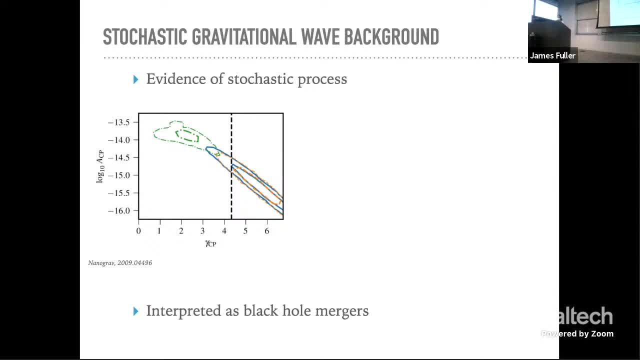 I wanted to add one more comment, because I'm throwing hooks out. there is that, even though you know, from a Occam's Razor point of view- perhaps the most likely one is the astrophysical one- dark sectors actually also would generate a signal that could look like: 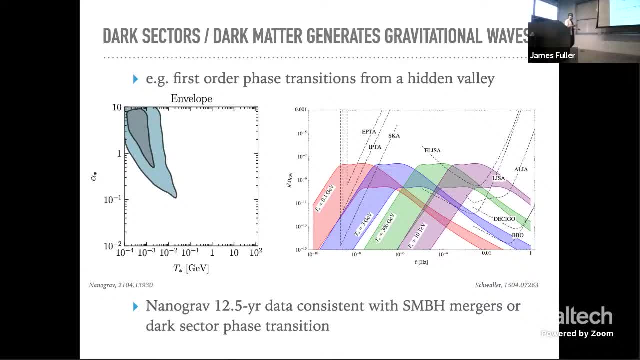 this. So the idea is that some something that would be analogous to the QCD phase transition, but strongly first order, could generate gravitational waves. Depending on what the temperature of that phase transition is, you'll generate different frequency gravitational waves And it'll have an amplitude that in general, 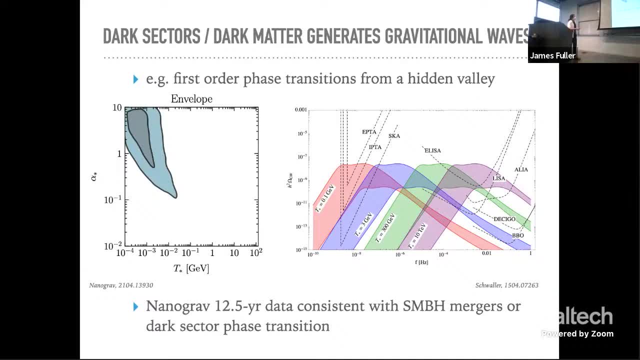 is large enough to be observed, either with PTAs if the phase transition is low enough, or, for example, with LISA at higher frequencies, higher temperatures for the phase transition. So you can go and ask the question: is the nanograv data equally well fit by a hidden sector phase? 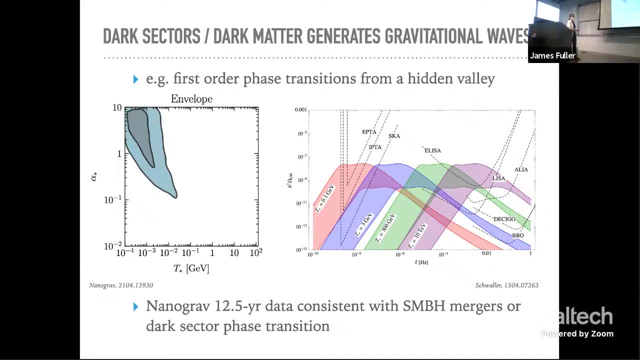 transition, And the answer to that question, at least right now, seems to be yes, That in fact you can generate that stochastic gravitational wave background with a phase transition temperature around one to 10 MeV, And then this is a parameter. 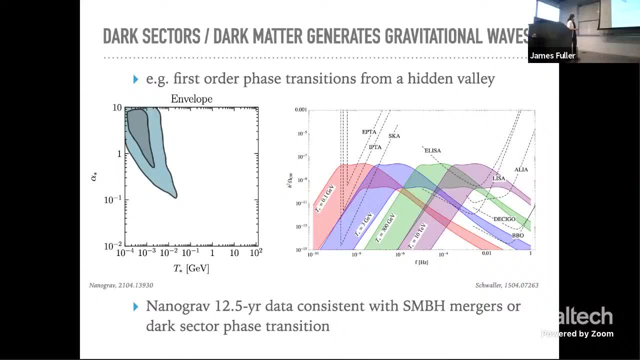 that tells you about the strength of the gravitational waves of the phase transition that's generating the stochastic background. So we'll have to see, as time goes on, get more precise frequency information, whether one can actually distinguish between an astrophysical source of such a background and a new physics explanation of the background. 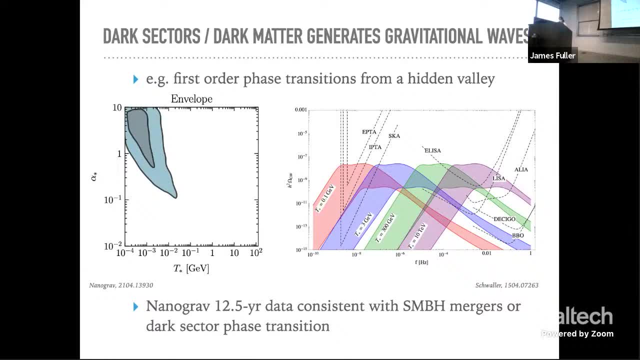 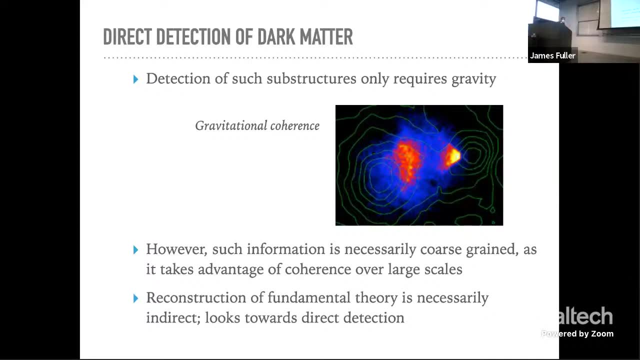 So that's all I'm going to say about PTAs, And I would just like to remind you that everything that I've said so far is utilizing only gravity, And what we're taking advantage of is gravitational coherence. So you're making these measurements. The question is really: how well can I weigh two objects? 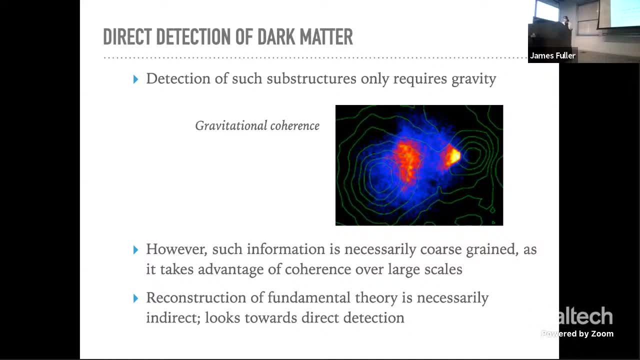 and look for the formation of structure on some scale. However, this information is necessarily coarse-grained, as it is at the root. It's really complex for the brain structure And so, if you're, it has to take advantage of that coherence of summing over many, many dark matter particles. 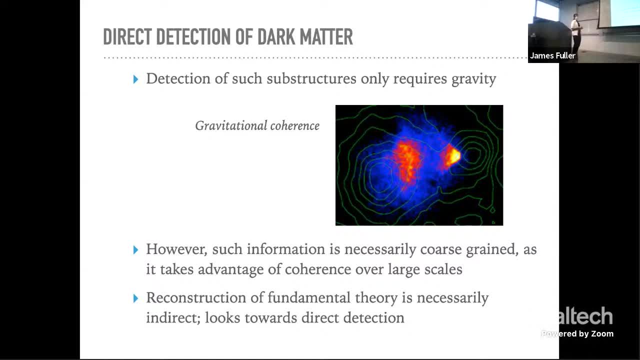 to be able to get a signal that's large enough to be detected through a mediator, which is the gravitational force. The reconstruction of the fundamental theory is necessarily indirect, So it might be the case that if, eventually, you can reconstruct the halo mass function to small scales, that you'll be able to determine what the theory of dark matter is. 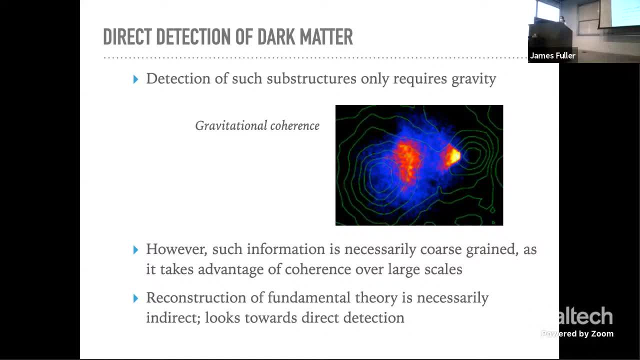 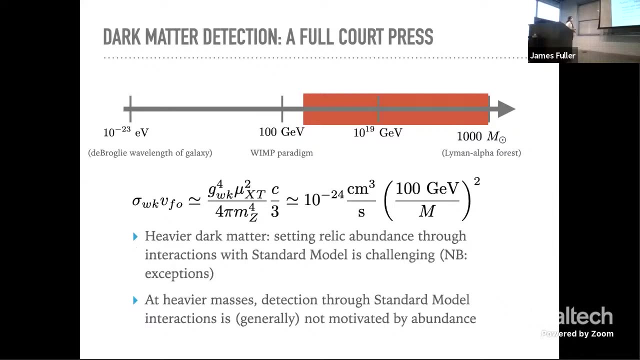 But you're not going to be able to detect an individual dark matter particle this way, You're not going to be able to reconstruct the Lagrangian, the fundamental theory, the kind of information that particle physicists want for a complete theory. So I'm going to now come back to my earlier picture, because I want to transition into 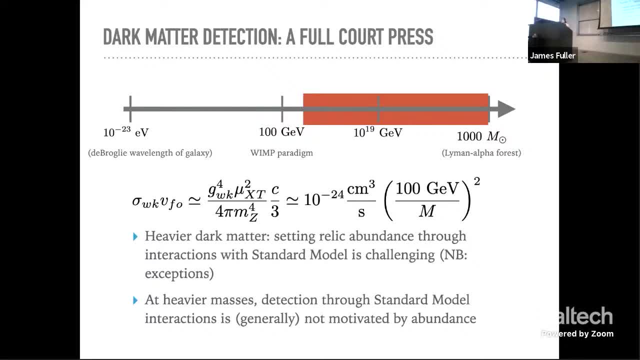 talking about the particle interactions of dark matter and ways that we could look for those. So I want to start on the high mass end. So before we were looking at this window from about an MEV up to the TEV scale, And once you get above a few TEV and you're looking at this window all the way up to about. 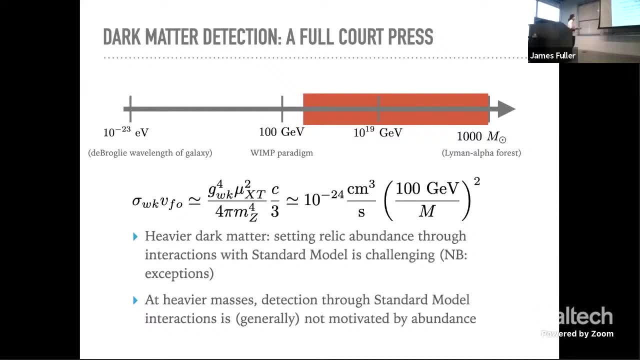 a thousand solar mass. setting the relic abundance in this window through the interactions with the standard model is challenging And the reason for that is again coming back to our back of the envelope. Estimate the weak this rate for setting the relic abundance. 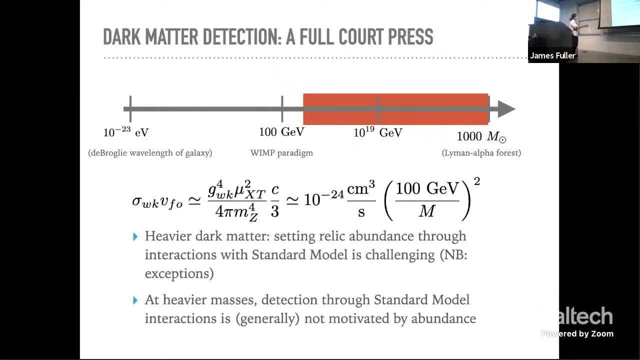 Now, if we just take this cross section and we look at it as you push this mass scale up, this drops, and remember the number that we needed to set the relic abundance was three times 10 to minus 26 centimeter cube per second. 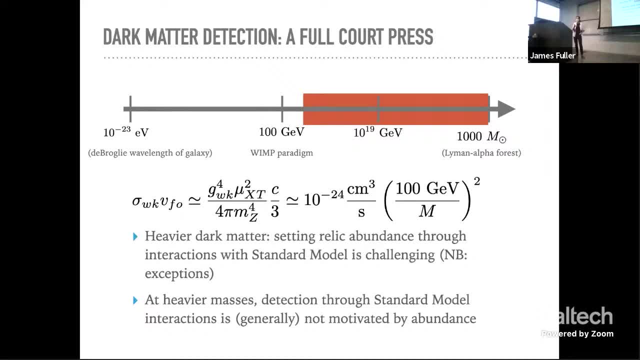 So once this process, this mass scale gets much above a TEV, you just can't set it through the interactions with the standard model, at least not at the dark matters. thermalize, So In heavier masses, detection of this dark matter through the interactions with the standard. 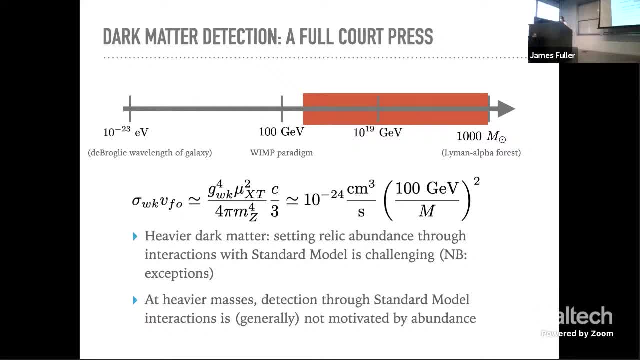 model is generally not that well motivated. Okay, So, so we want to still look for astrophysical ways to determine something about the nature of the dark matter at these higher mass ranges. And I want to give you one example of this because, because it's fun and quite generic. 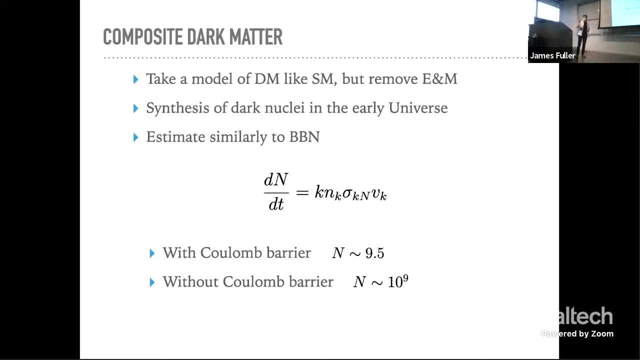 Okay, So let's imagine that in the hidden sector, I had a copy of the standard model, but I removed electromagnetism. Okay, This is would be actually totally consistent with what we know, But it would have a radical change in what we would see in the universe. 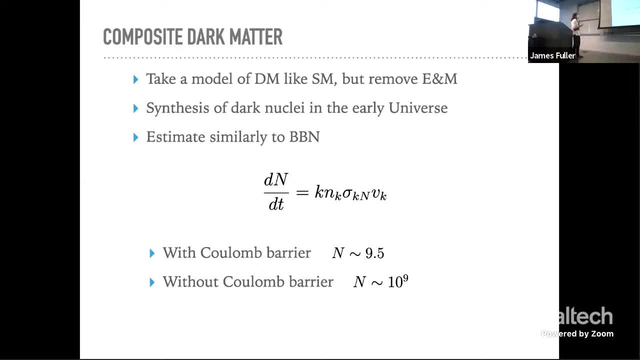 And I just want to do a little, another little back of the envelope estimate. So we know that the standard model nuclei, at least the light ones, are synthesized when the universe is a second old at BBN. Okay, And so when you learn about BBN and taking your class, what you do is you solve a Boltzmann. 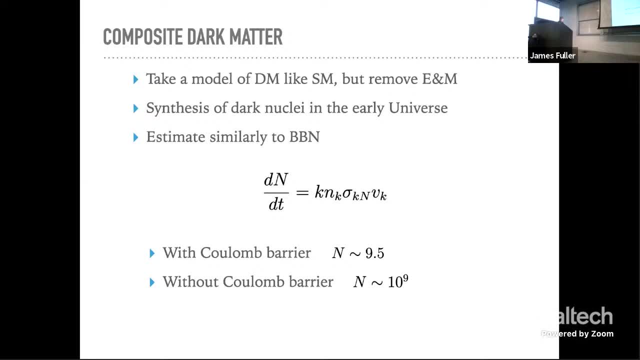 equation where you say that the synthesis of an of an element of size, capital N, goes like some cross section, usually geometric cross section- times a relative velocity and then the number, density that's available and there's some order, one number here. Now, if you put in a cross section, that's relevant to the standard model which is dominated. 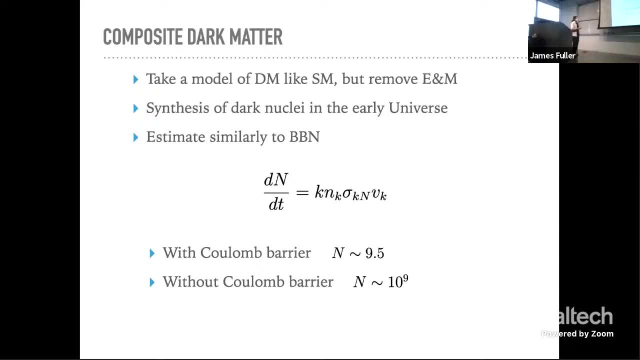 by the fact that there's a coolant barrier, You synthesize nuclei. if you just do this simple back of the envelope, which is about nine and a half, And it's pretty darn good because we know in BBN we synthesize lithium seven but nothing. 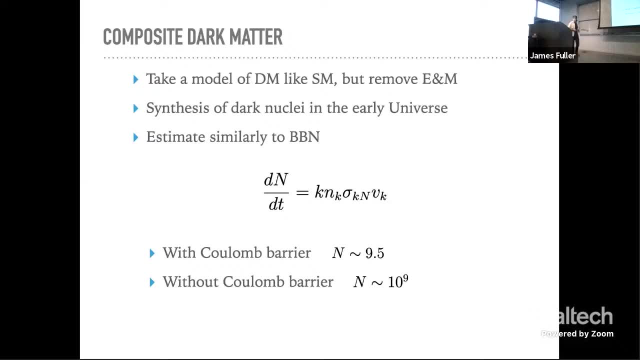 larger. So now let's just get rid of that coolant barrier and otherwise have the standard model physics proceed as it would. otherwise, what do you synthesize? you synthesize, actually, huge nuclei, Right? This would be completely consistent with what we see in the universe. 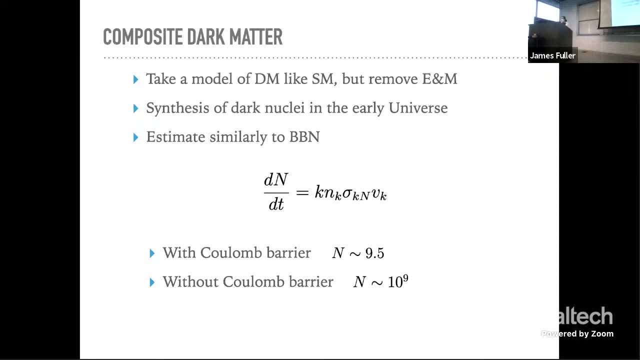 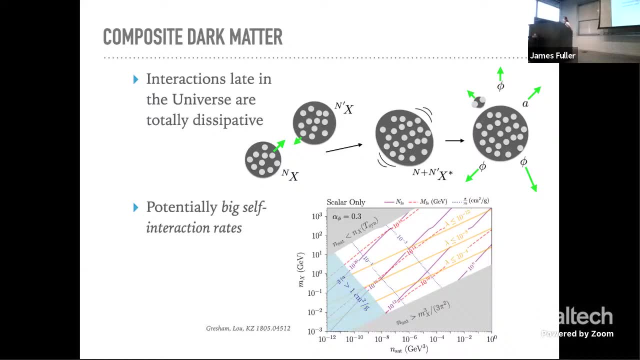 Okay, And the and the consequence would be that you would have these huge nuclei sitting around. their cross sections would be large and they would play generically interact with each other And when they interact They, just like in the standard model, they would stick together. 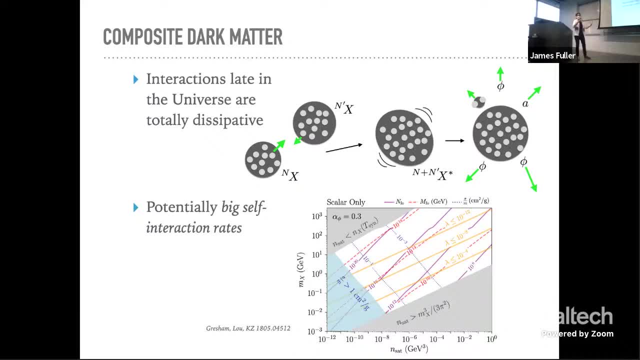 They would fuse, it would be a maximally dissipative process- and then they would bring down to the ground state by radio force mediators. so in the standard model these are pions. If you have some hidden sector, this would be an analog of pions, which here we call a scalar. 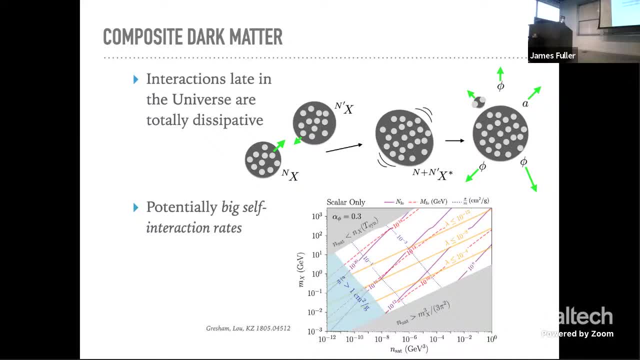 five, And so you can, you know, just ask this question and then compute what the model space is for this, And it turns out that there's a significant part of the model space where the interactions would be astrophysically relevant. 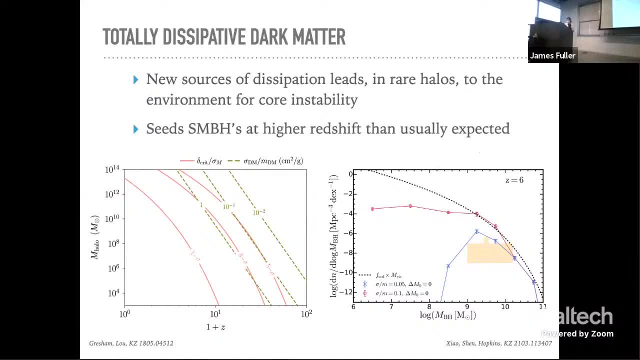 And it would lead to new sources of dissipation and halos and potentially to core stability. Now, in general, we don't see halos destabilizing, but we also know that we have a population of halos, so not all halos do the same thing. there's a great diversity and the halos that 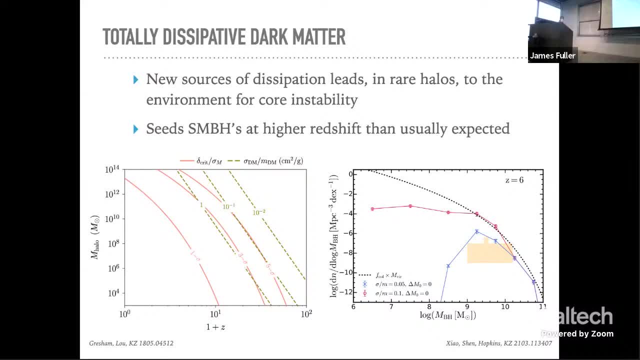 we observe in the universe. So one thing you can think about is that we don't actually know how supermassive black holes are formed in the very early universe at redshift save six. So one thing you can ask is whether this type of dissipative dark matter 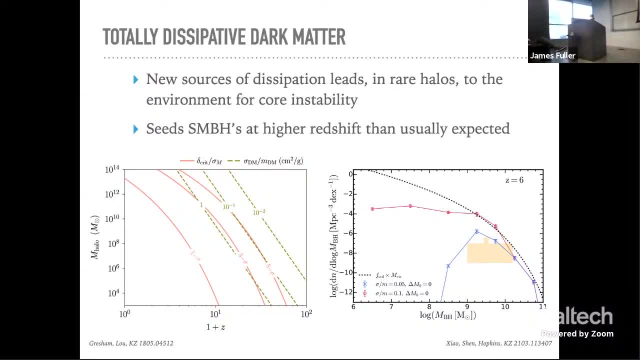 Okay, Could cause an instability that would see supermassive black holes in the early universe, but would still be consistent with what we observe at low redshift. And in order to look at this, what needs to happen is that you need to have massive halos. 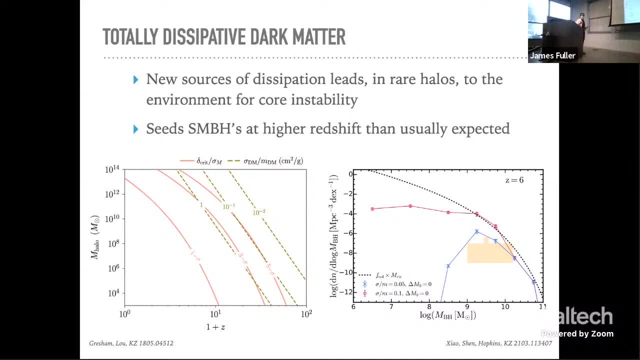 that at high redshift would destabilize, but they should be relatively rare, high density halos And that actually allows you to fix a preferred interaction cross section for this process. So then you can look at the hill, the halo mass function of the supermassive black holes. 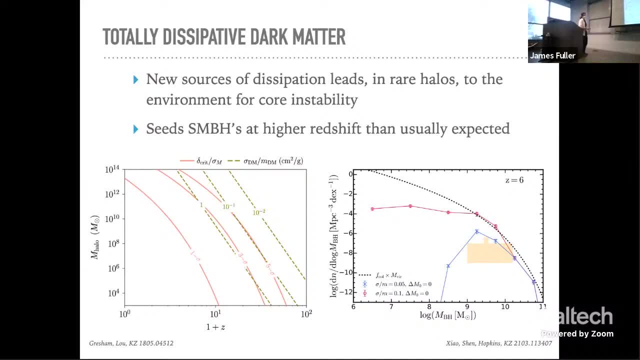 Okay, at, say, 10 to the nine solar mass that you would like to understand, at a redshift to six, and see whether this type of dark matter model could quite easily and naturally do this. So, Phil Hopkins student, Jacob Shen, and another student who's working with me, Huangyu Xia, 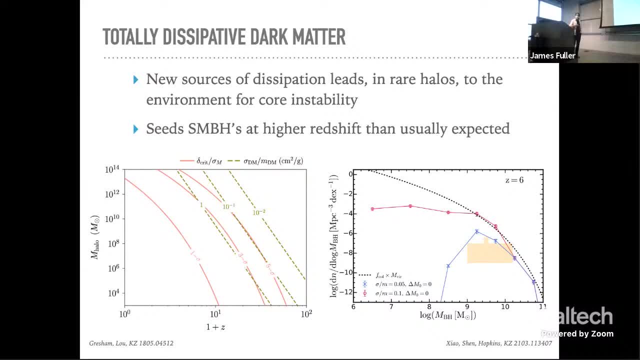 looked at this and it turns out- I think there was maybe some skepticism initially, but this actually works quite nicely to see the formation of supermassive black holes in the early universe. So, backing up for a minute and thinking about models of dark matter that are quite simple, 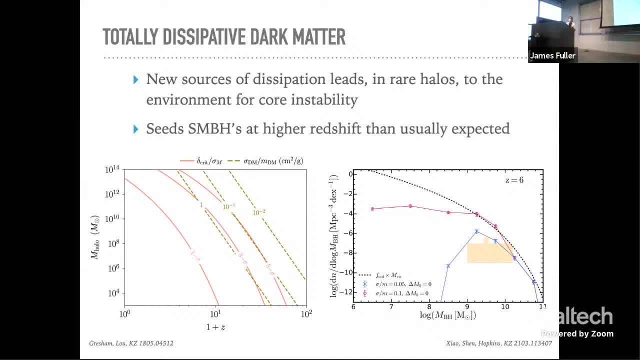 to construct from a theoretical point of view, but are not the standard WIMP can actually give rise to radically different astrophysical predictions, And so You'll always be asking yourself this question: how much am I biased by the CDM paradigm, where 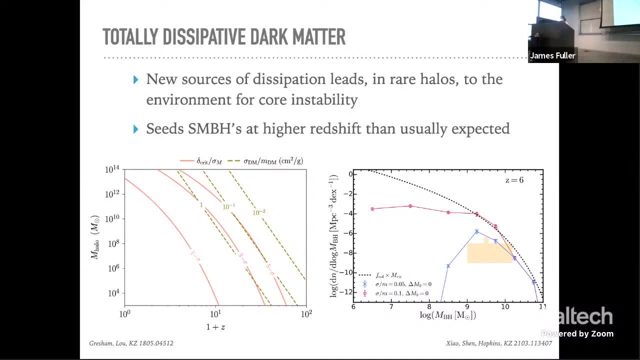 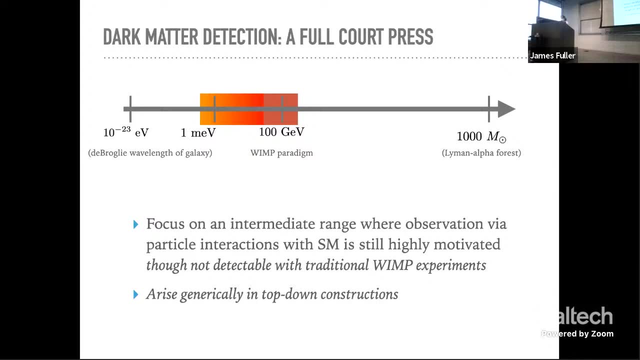 there aren't any relevant dark matter dynamics. Okay, So in the remaining time I want to talk a little bit about direct detection. So I'm coming back to this plot. So I said up here the internet, it's really not very motivated to look for dark matter. 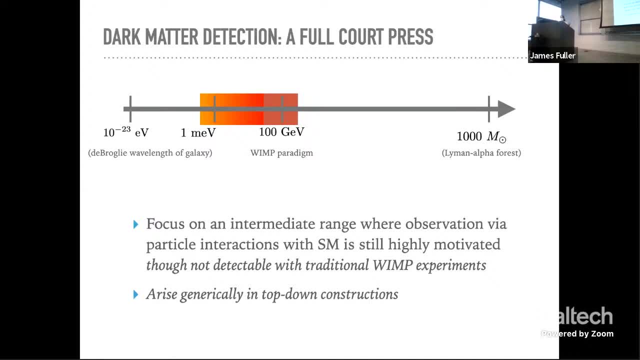 through its interactions with the standard model, Through its Relic abundance, because the cross sections are just too small, They're suppressed by one on the mass squared And in general, at least from the relic abundance point of view, not really motivated to look. 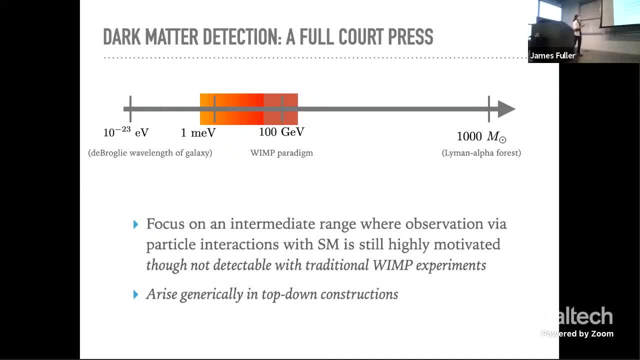 in direct detection experiments. On the other hand, if you go to slightly lower masses, the cross sections can actually be enhanced relative to the weak scale cross sections, but they're actually not detectable with the suite of experiments. So I'm going to talk a little bit about direct detection experiments that were designed to 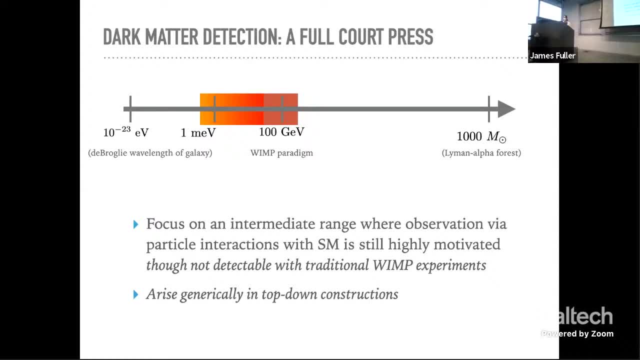 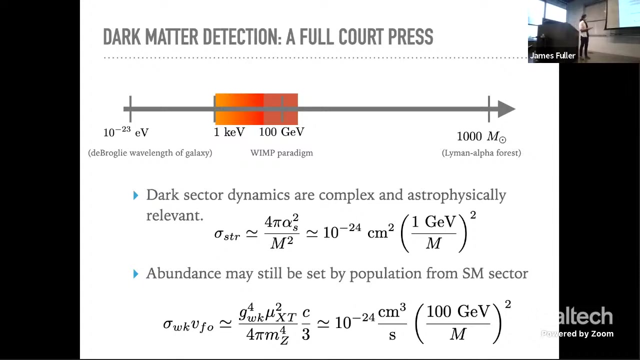 look for dark matter at the weak scale. So there's a giant hole in looking for these low mass hidden sector dark matter models, And I want to emphasize that these models arise generically in top-down constructions. Okay, So to make another, to make this point again, the dark sector dynamics are complex and, astrophysically, 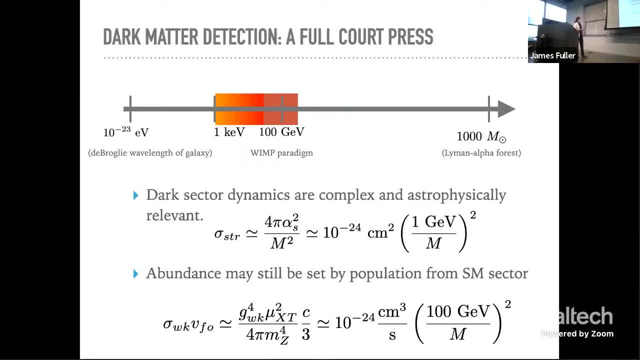 relevant. So The interaction Cross-section- now again doing the naive dimensional analysis estimate, turns out to be about 10 to the minus 24 centimeters squared if the mass scale is around a GEV. So this is a cross-section that again would be on the scale that would modify halo shapes. 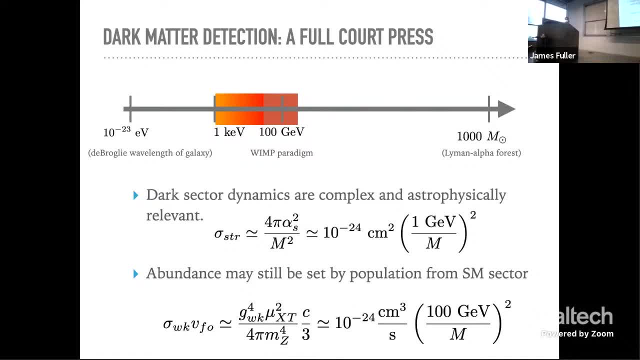 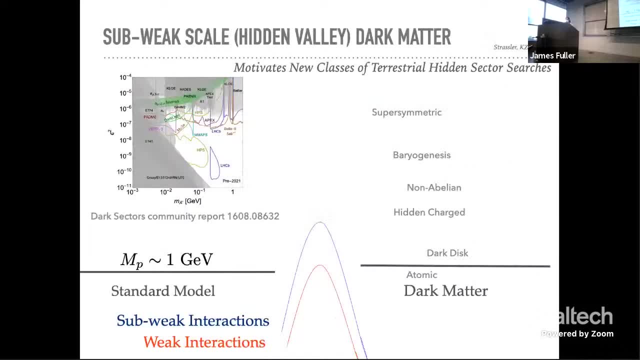 and the abundance can still naturally be set by the interactions with the standard model, And so this motivates new classes of terrestrial Hidden Section Sector searches. So 15 years ago none of these experiments existed. Okay, People weren't thinking about this. but in the last five years now there have been. 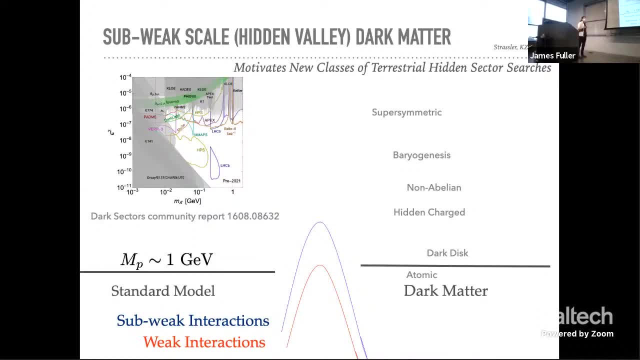 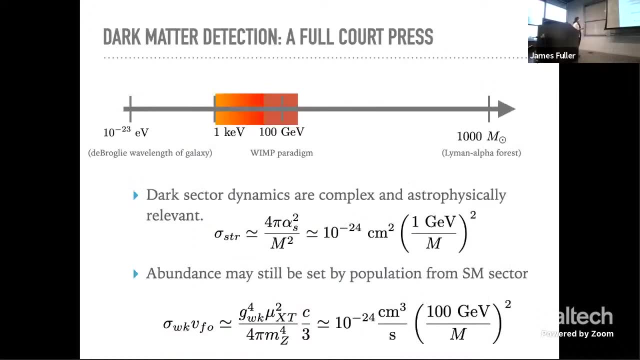 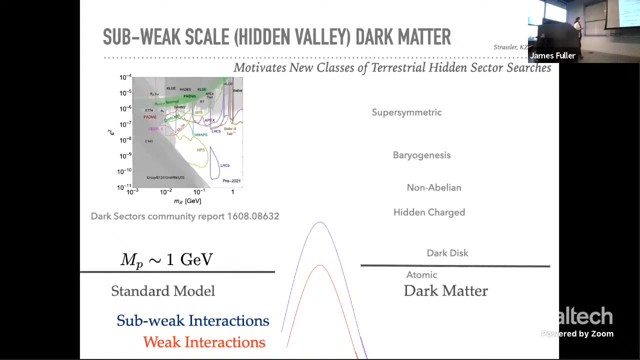 a suite of experiments in colliders and also in direct detection that have been designed precisely to look for dark matter with mass just below the electroweak scale, And it would be a lot of fun to spend some time talking about these accelerators. 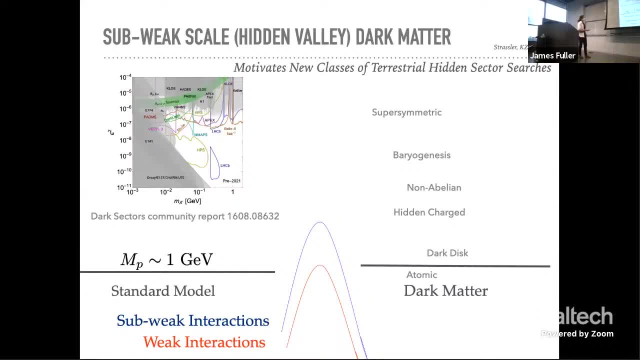 Okay, So we're going to talk about these accelerators. So let's start with the accelerator based searches that are looking for dark matter, hidden sectors by relatively low mass mediators, But again making it an editorial choice, We're not going to talk about that. 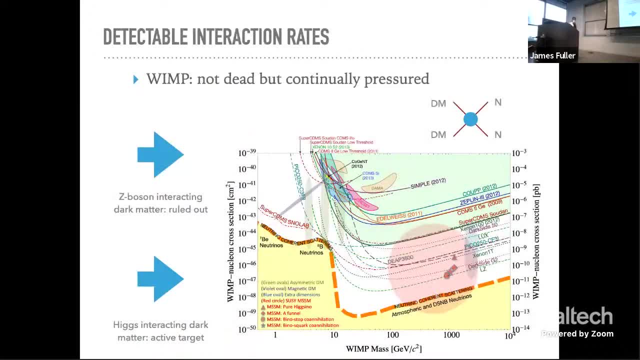 We're going to focus on direct detection experiments. So the direct detection experiments that look for the WIMP Focus on a process where dark matter scatters, elapsed elastically off of nuclei and deposits a significant fraction of its energy. Okay, And one of the reasons why that works well is because weak scale dark matter is actually 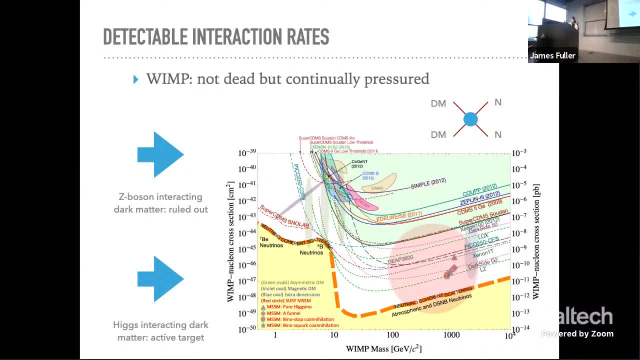 kinematically well matched to nuclei. So if I have dark matter, which is say a hundred GV to one TV, typical heavy nuclei are around a hundred GV, And so it turns out that that is a good kinematic match for extracting a lot of the dark matter. 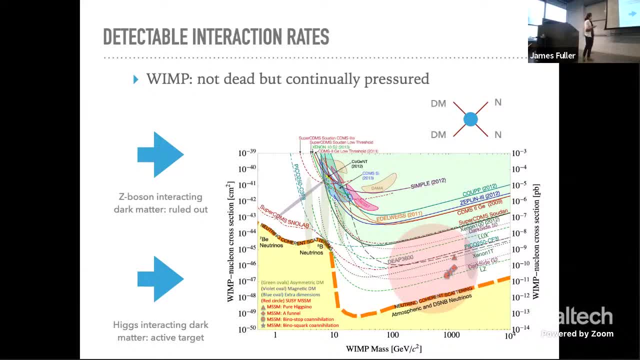 kinetic energy, And so these direct detection experiments We're going to look for dark matter interacting with nucleons through some procession is a function of the dark matter mass, And so these sets of curves. I want to draw your attention to two things. 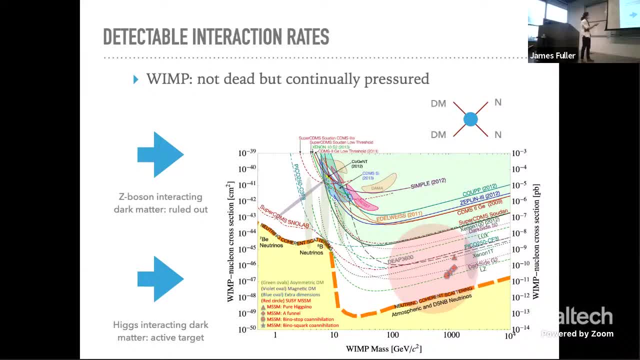 First of all, the Z bows on that. typical interaction cross-section is 10 to the minus 39.. This is where the experiments are right now. They're actually at the 10 to the minus 46 centimeters squared level. So that has been ruled out by many orders of magnitude. 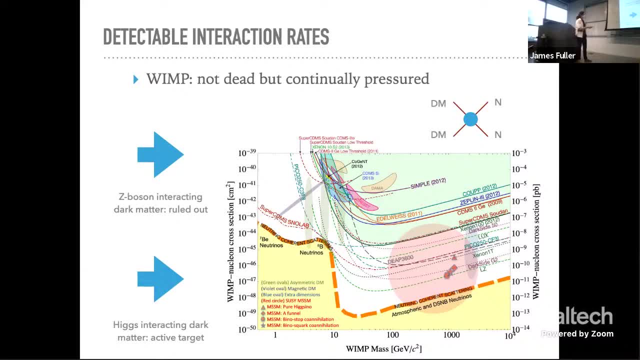 Okay, What these experiments are probing right now is the regime where dark matter interacts with the standard model via the Higgs, And that is kind of this bullseye, strictly speaking, it actually doesn't close, continue downward, but eventually we're going to hit in the future, looking beyond LZ, which is 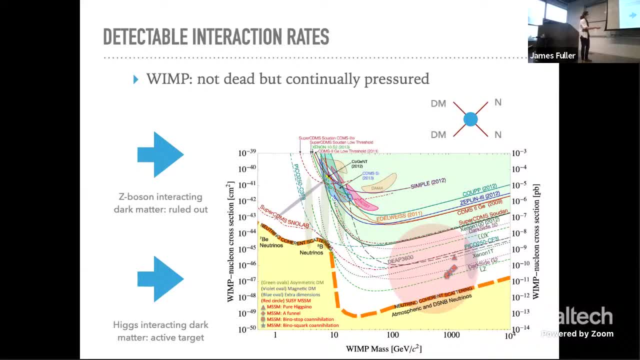 a Xenon experiment based out of LBL. we're going to hit the atmospheric and solar neutrino backgrounds And once you get to that point you don't get linear scaling anymore. You have to now deal with the background of the solar neutrinos and the experiments become 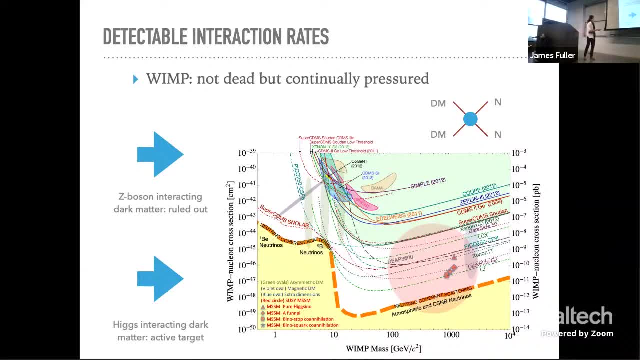 very hard. So many people view this as being kind of the practical limitation. On the other hand, you can see that all these experiments have no sensitivity with mass below 10 GeV, And that's partly to do with the way these experiments are. well, it is to do with how 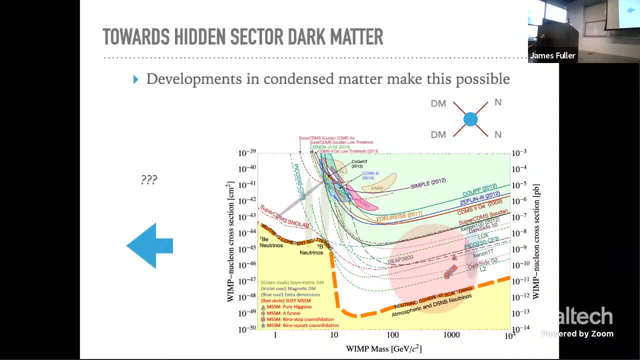 these experiments were built, but it also has to do with the theory bias that went into that, Which said we don't need to look for dark matter much with mass much below 10 GeV, And so there's been a movement to ask the question: how do I look for dark matter hidden? 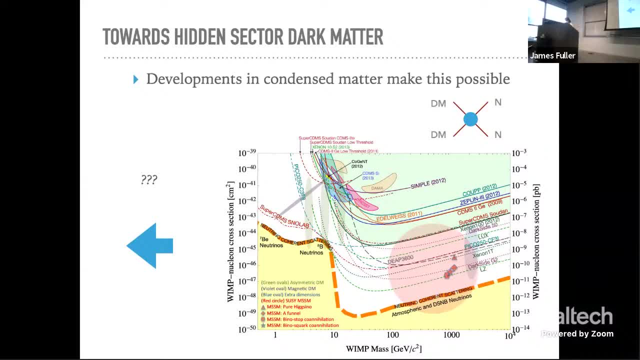 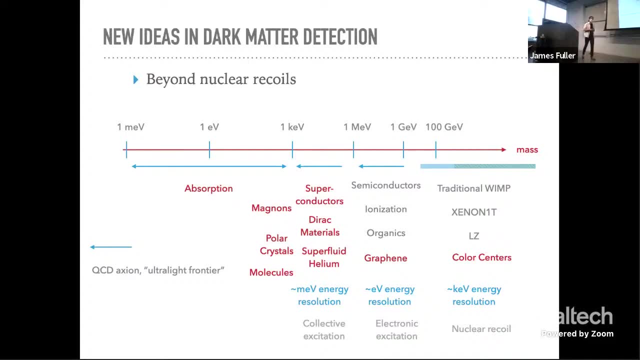 sector dark matter at these much lower mass scales. So fast forward to 2021, okay. And now we've had an explosion of ideas And some of these. you know we're going to have to look for dark matter at these much. 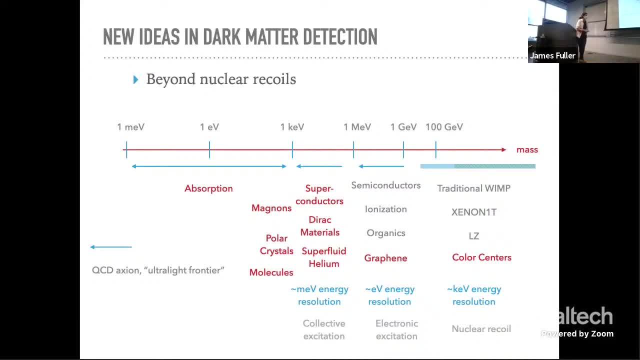 lower mass scales And some of these. I'll talk about a few of these, the ones that I think are most likely to succeed. Okay, And why I think that's the case, But what I want to highlight here is- again- I'm looking at this window- MEV dark matter. 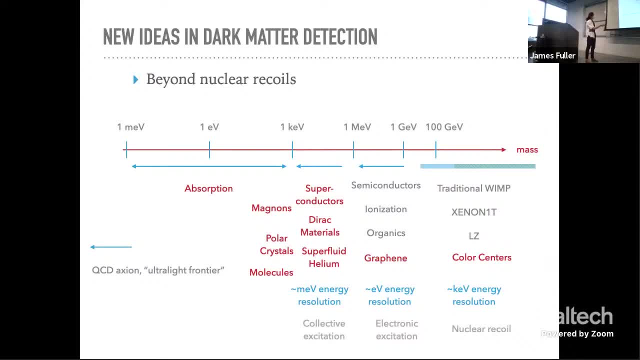 So here's the weak scale. you have the traditional WIMP experiments, you go down another three orders of magnitude and you want to look for electronic citations? okay, with now three orders of magnitude. So this is the ability of the EMI to measure the magnitude improvements in your energy. 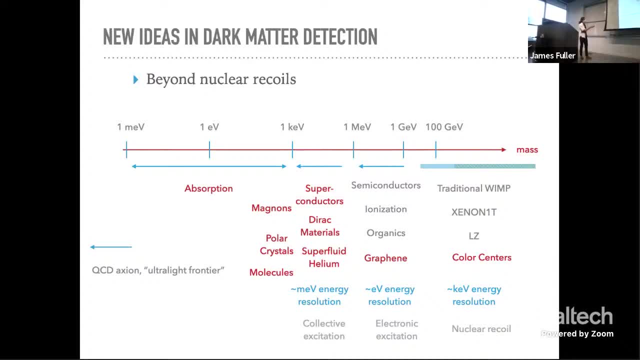 resolution And then down to a KEV. this is basically where dark matter can be populated in some way, not thermally, but in some way. this interaction with the standard model. Now you need millie. the energy resolution and the relevant excitations are collective. 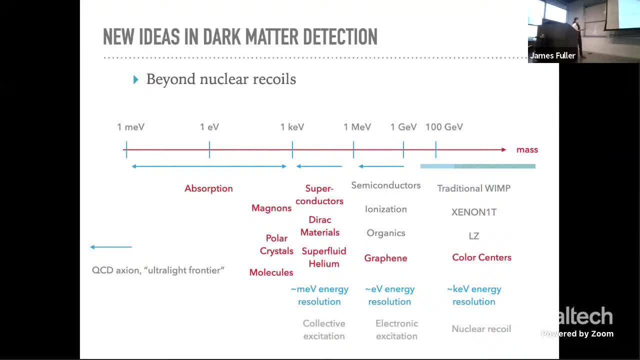 excitations, And this really covers the entire mass range where the abundance being set by its interactions with the standard model is relevant. So that's really what we're looking for. Okay, So now we have a little more. So now we have a little more data. 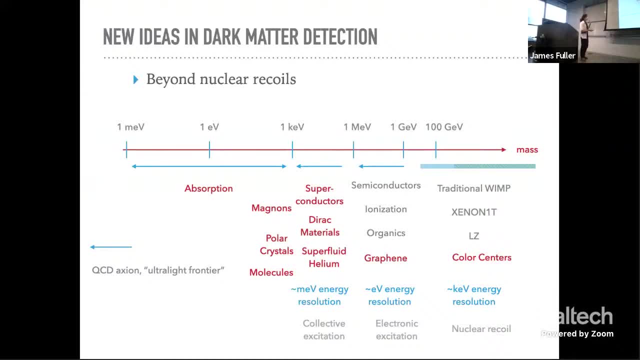 Okay, so you're. with these combination of technologies, you're going to get a huge number of dark matter candidates that you're sensitive to. I want to also comment that for every order of magnitude that you get up here above the KED, you get another order of magnitude for free. 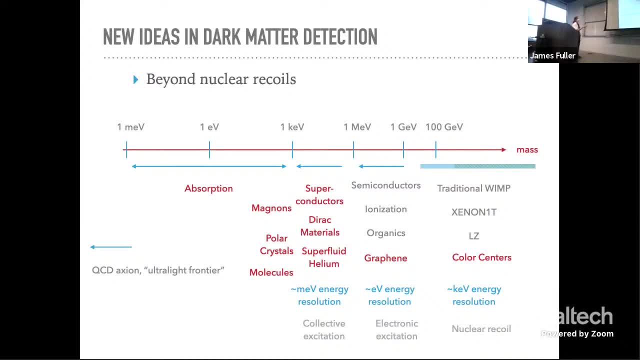 This is: you're depositing the kinetic energy down here, you're depositing the mass energy. So combined, these experiments are going to hit 12 orders of magnitude in dark matter mass. And because we're taking a shot in the dark, you don't want to be in the dark anymore than you have to be. 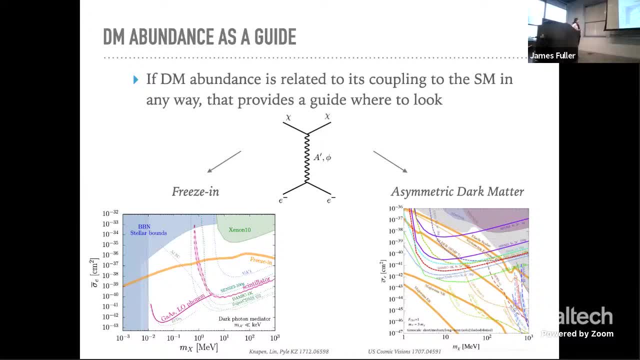 You should have a theory that is motivating your search. So, to come back to an idea that I said earlier, the dark matter abundance is really providing that guide. So when the dark matter's abundance is fixed by its interaction with the standard model, then that will predict a scattering cross-section. 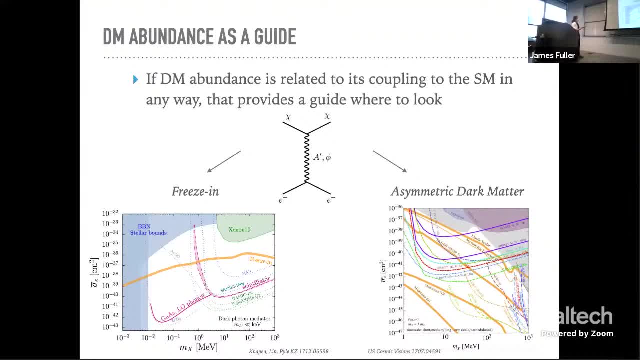 So if I have some process where annihilation, say, allows the relic abundance to be produced, I just turn the diagram on its side. There's a crossing symmetry and it predicts a direct detection cross-section. So here's the interaction cross-section as a function of the mass. 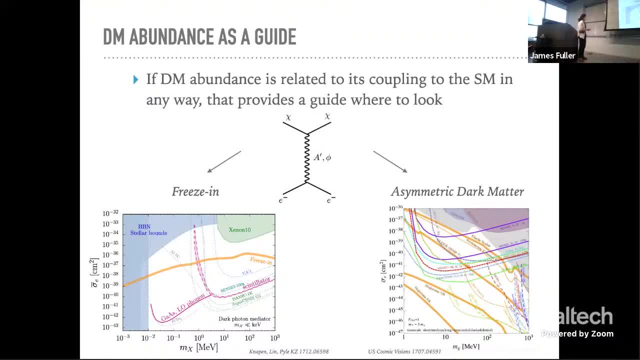 There's a lot of detail in these plots. The point that I want to make is that there's these orange bands, And the orange bands correspond to regimes where the interaction with the standard model produces the relic abundance that we observe. So it fixes that. 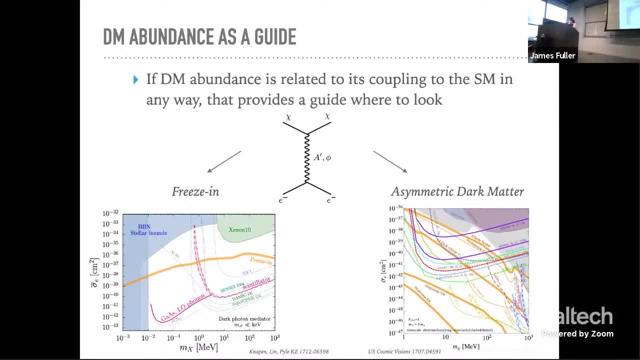 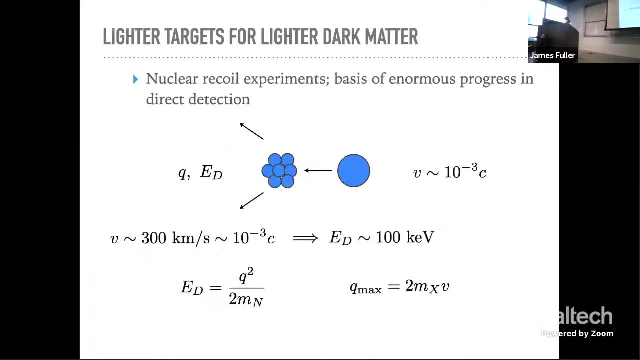 So this is the interaction cross-section in that class of models. So how much time do I have left, What? OK, So let me race through this and just tell you if you're going to get another 12 orders of magnitude in mass. 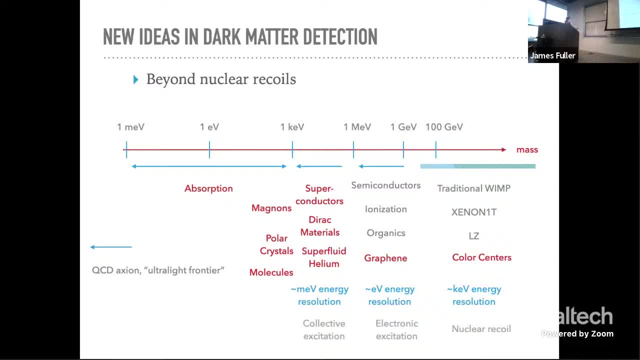 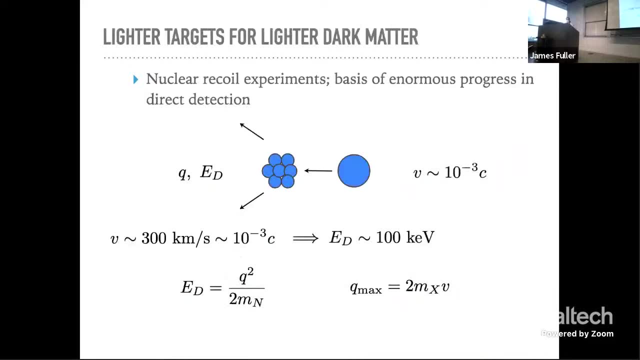 so you're going to go from the traditional WIMP down to electron volt sensitivity, down to milli electron volt sensitivity. what is it that you have to do in terms of the ideas? So nuclear recoils literally work like a billiard ball experiment. 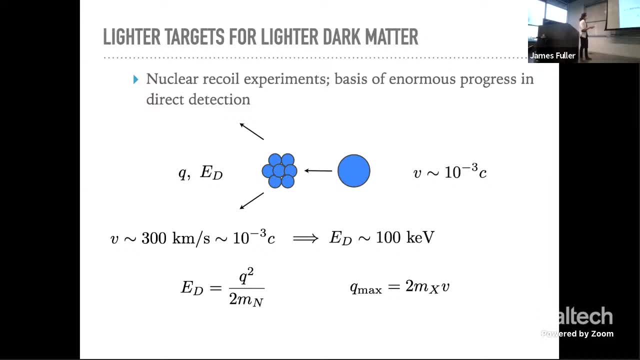 Dark matter comes in, It scatters off the nucleus, It deposits this kinetic energy And you can do the non-relativistic kinematics problem And it turns out that the deposited energy is in the 10 to 100 keV range. 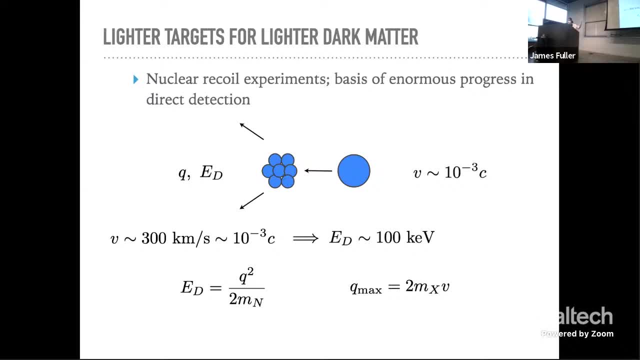 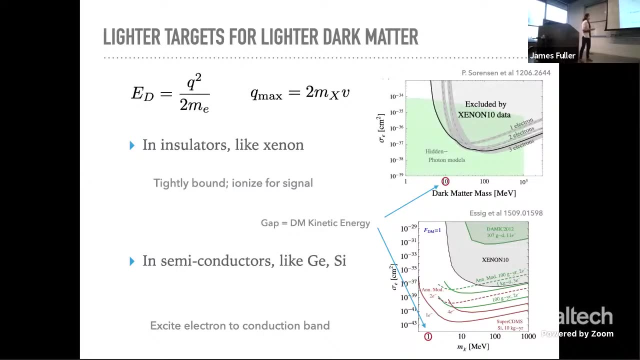 And this fact is what really motivates the experimental choices For direct detection of dark matter through elastic scattering off of nuclei. That is appropriate for weak-scale dark matter, If you want to go down the next three orders of magnitude, down to MEV mass dark matter. 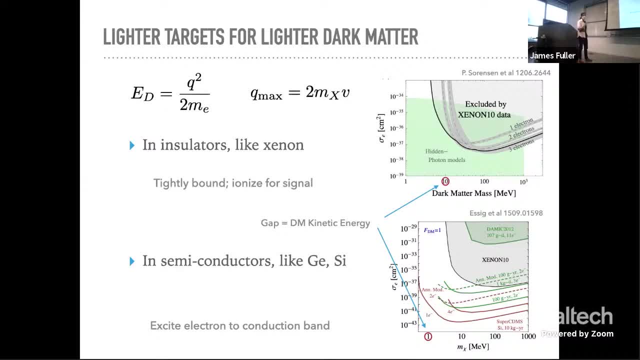 then you actually need to look at later targets in order to be able to extract more of the dark matter, kinetic energy. So again, stating it very simply, the energy deposited is the momentum transfer squared over the electron mass. And you know, the most amount of momentum you can transfer is MEV. 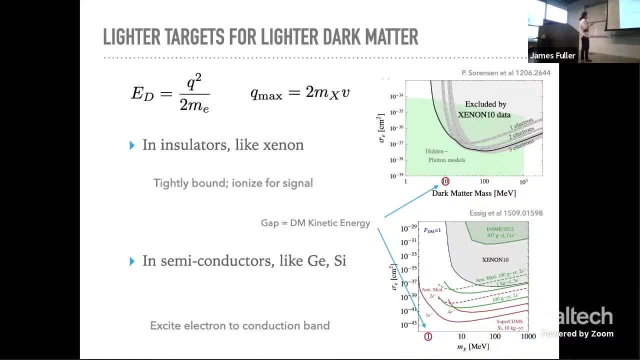 And so now you work that out And MEV, dark matter will deposit at most an electron volt of energy, because dark matter is moving at 10 to the minus 3 times C, And so that means good places to look are an ionization of electrons that has about a 10 electron volt gap. 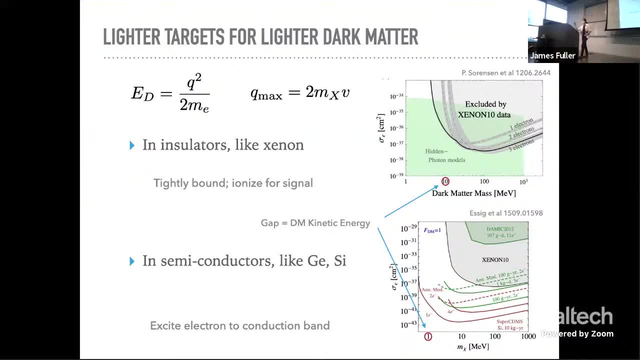 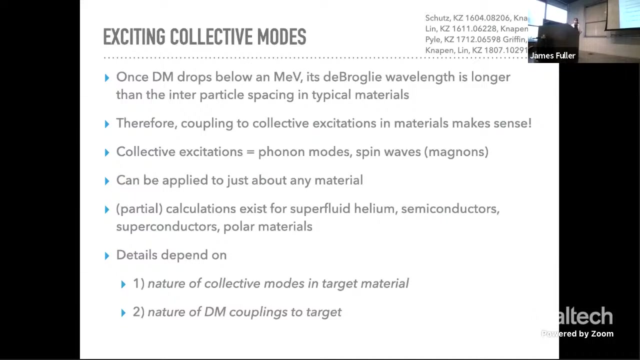 or excitation of electrons from valence to conduction band That has about an electron volt gap. If you have dark matter now that is dropping below this MEV mass scale, then you have to think about new things entirely. And this is where you start to realize that, unlike in nuclear recoil experiments where you treat the nucleus as being free, 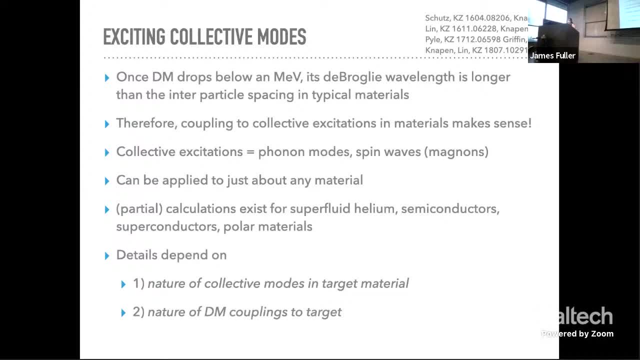 when you look at a nucleus in a typical material, it of course is not free, And in addition, when the dark matter mass drops below an MEV, its de Broglie wavelength becomes longer than the inter-particle spacing. So that means that I don't just interact with one nucleus or one electron. 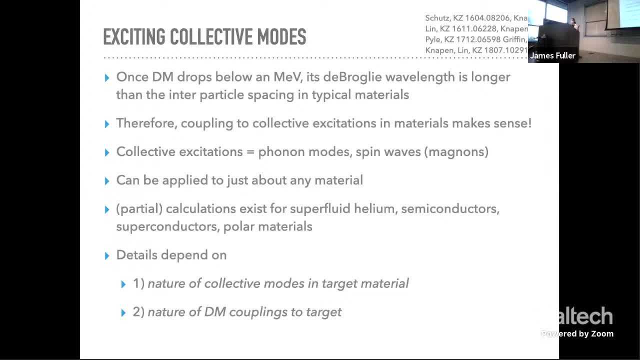 I'm actually interacting with the lattice- The degrees of freedom in the material change, and I need to compute the excitation rate for collective modes, And I would love to go through the details of that, But I think I probably don't have time. 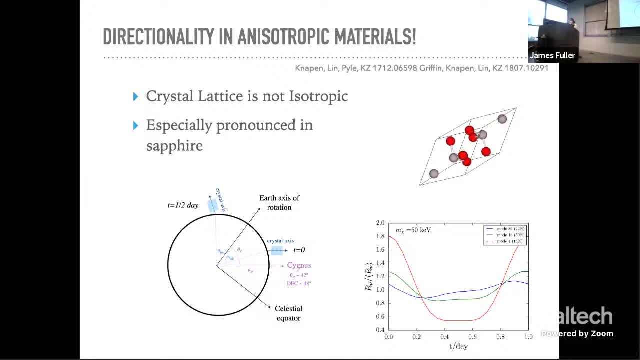 So I'm just going to skip ahead and show to you. Well, I want to say one more thing. that's really cool about this is that you get directional detection. So the Earth- that's what this is- points to the dark matter, wind. 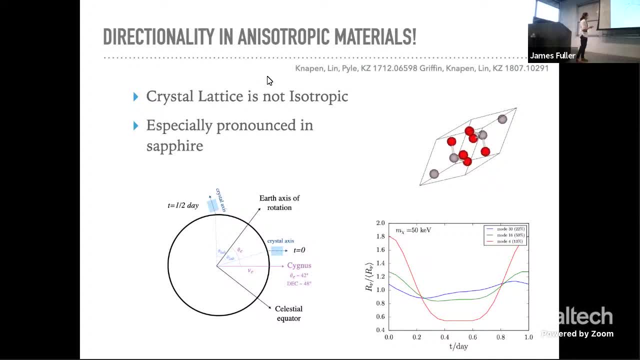 Dark matter. wind goes towards sickness, And the Earth is oriented with respect to sickness At some angle. I think it's about 43 degrees, if I remember right. And so, as we rotate on our axis, the orientation of a dark matter detector with respect to the wind is going to change as a function of the times of day. 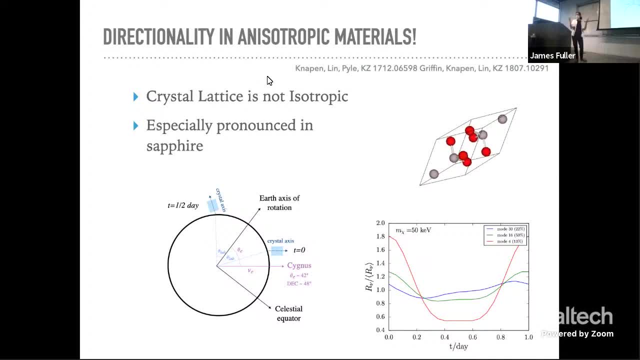 And now when I have a process where I excite collective modes in the material, those collective modes are not isotropic, So this is completely different than the standard nuclear recoil case. I have excitation rates now that depend on the time of the day, because it matters whether the dark matter particle is coming in this way and exciting the mode, or whether it's coming in this way and exciting the mode. 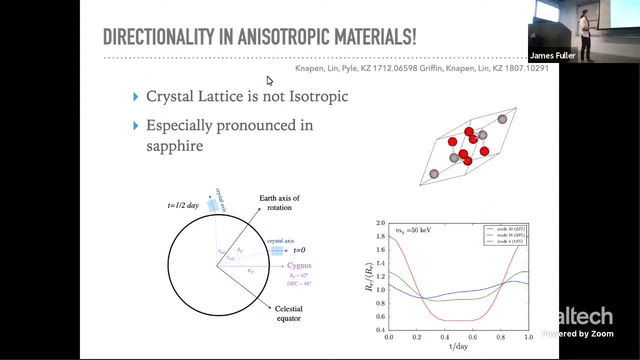 And this actually gives rise to an order- one variation in the interaction rate in the detector, And because it depends, in particular, on how the detector is oriented with respect to the wind, this is actually a smoking gun signature that would allow you to actually really determine that you're seeing dark matter. 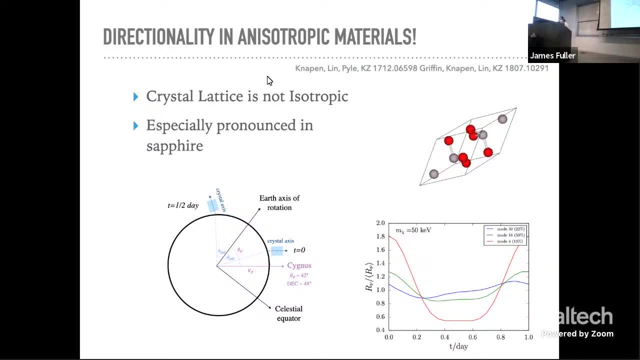 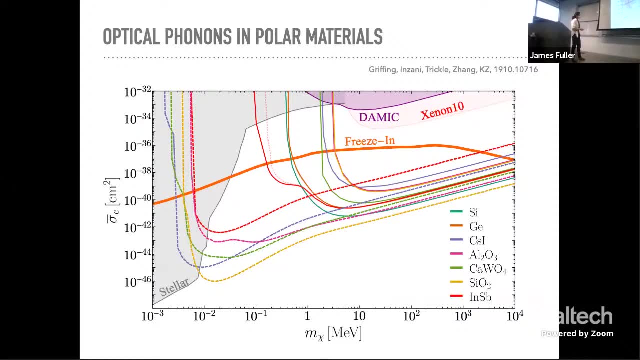 That you're seeing dark matter in your detector and not some other background. So this, these combination of technologies together allow you, through the scattering process now to get down to this KED mass window. So here I'm. you know this plot stops at 10 GeV. 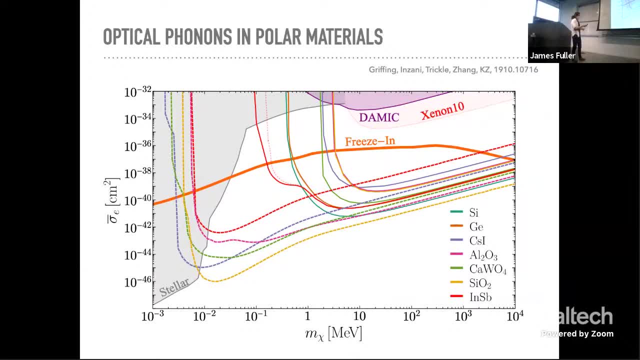 That's where the WIMP experiments pick up at higher masses And you can see that with now these detectors are a kilogram. Okay, You can see the Xenon experiments that are ton scale experiments is a very small experiments. You can cover some of these well motivated dark matter candidates by actually many orders of magnitude in the interaction cross section. 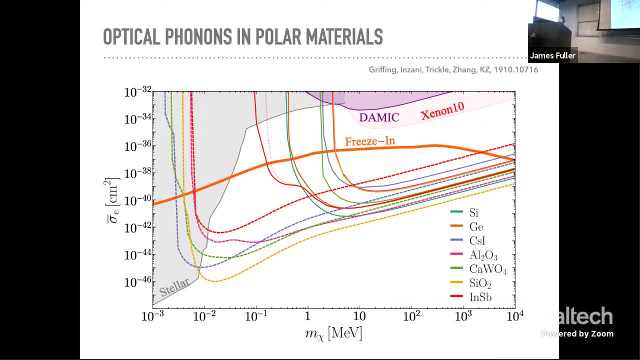 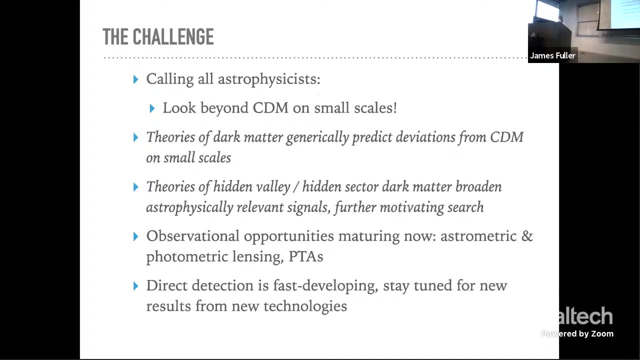 And so this is one of the major pushes within the dark matter direct detection community. right now, there are several funded experiments that are moving forward with this idea. Okay, so, let me conclude. Okay, so, let me conclude. So wanted to make this talk something of a call to really think about ways that you could make measurements of dark matter substructure with, in particular, halos that have densities which may not be typical of CDM halos. 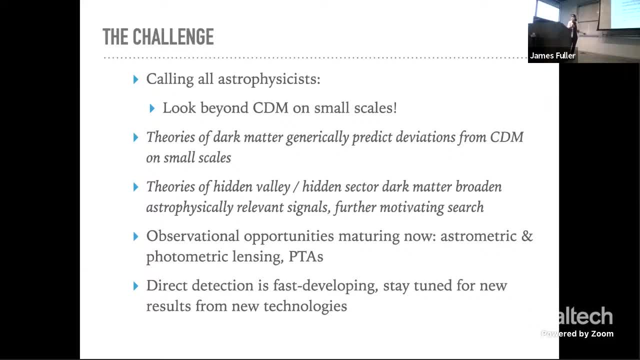 And you're not looking for strange models of dark matter. You're going to emphasize that this is generic, that on small scales you expect particle interactions are going to impact the formation of structure, And so you're. it's. it's not as if you're kind of trying to finagle with your dark matter model to give them kind of a signature. this just comes out naturally. theories of dark matter- okay, I already said this- theories of hidden sector dark matter in general. just 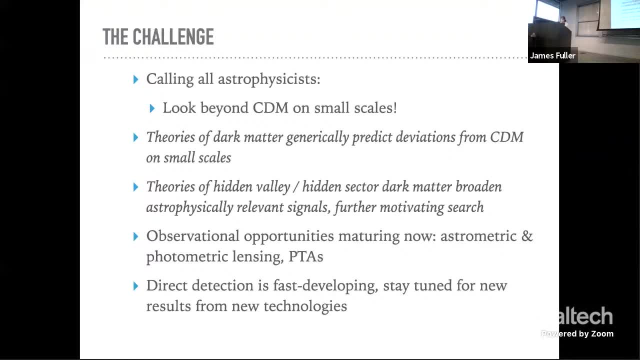 broaden the class of astrophysically relevant signals And there are opportunities that are to measure small scale structure that are maturing now. I think they deserve a lot more study. I mentioned just briefly astrometric and photometric lensing and pulse for timing arrays and direct detection. 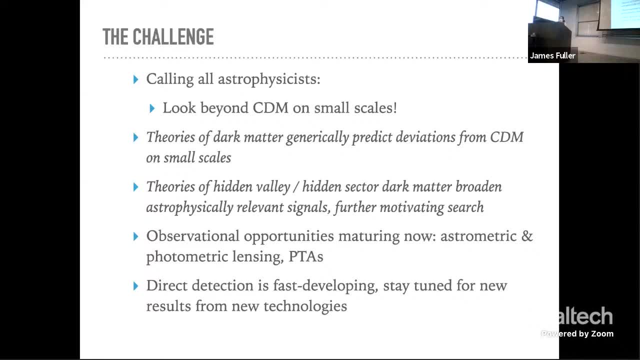 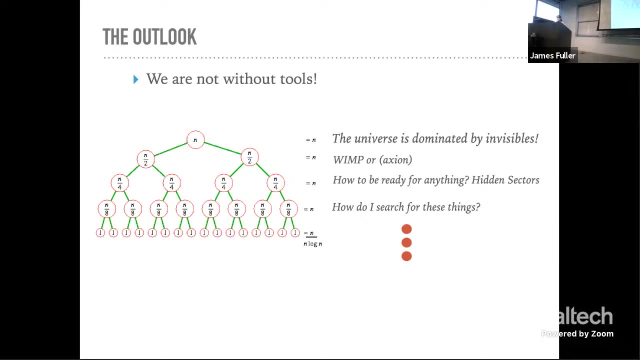 You know I didn't get to spend a lot of time on it- is becoming a fast developing area where people are pushing into this low mass dark matter regime, And so I My apologies- See me show this before, because I I often like to show this when I'm talking about dark matter, which is that sometimes, you know, you can get overwhelmed with the question of what is the huge problem, what is the nature of the dark matter. 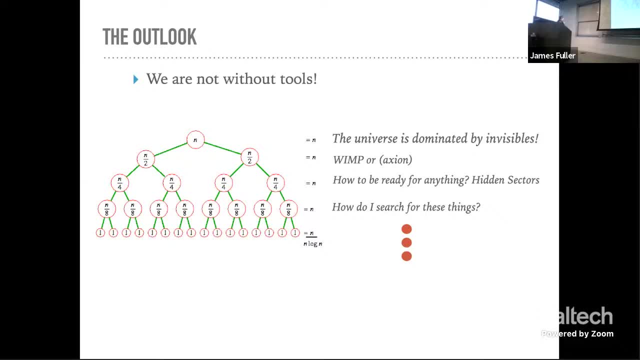 And we've made progress. We know that the universe has to be dominated by some physics beyond the standard model. We started with these ideas that the dark matter. We started with these ideas that the dark matter. We started with these ideas that the dark matter. 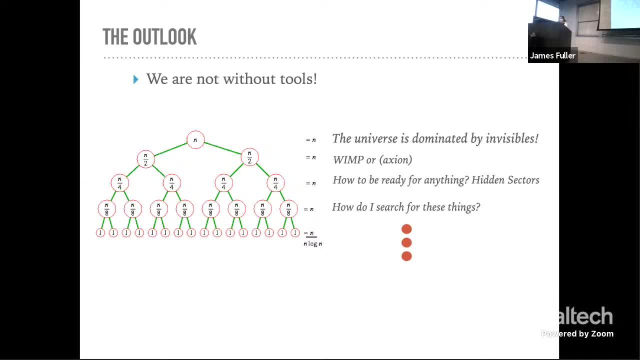 It doesn't have to be a lamp or an accent, or actually also, you know, black holes. We've really made progress on, you know, eliminating or strongly constraining those dark matter candidates, And so now we're thinking about dark matter in a way, actually, that is more can say analogous, the standard model, in the sense that there's dynamics. 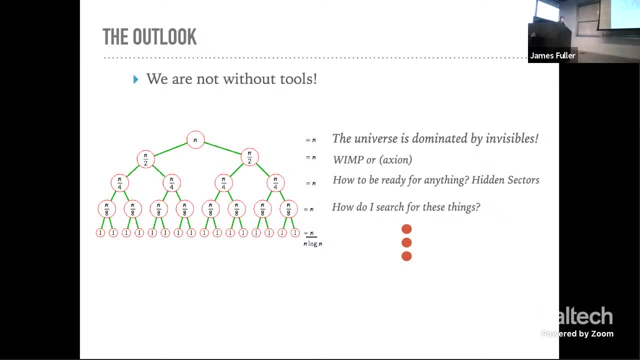 Okay, And so now we're pushing on this further and asking the question: okay, a broad set of candidates, how is it that I develop a broad set of tools to be able to look for all these dark matter candidates? So I think it'll be an interesting time. 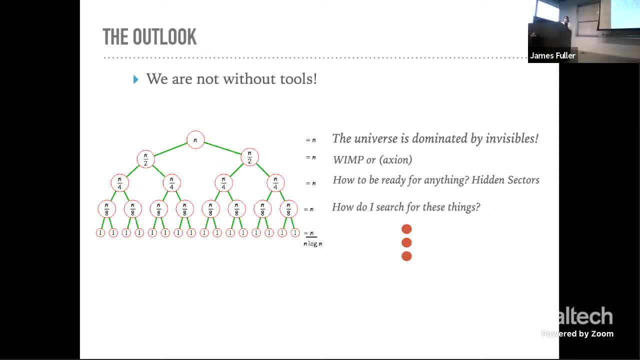 over the next decade to see how this evolves, And I'm certainly happy to talk more about that. So thank you, Thank you, Catherine, for that incredibly interesting and sort of rising, expanding view of this field, And so we have a lot of work to do. 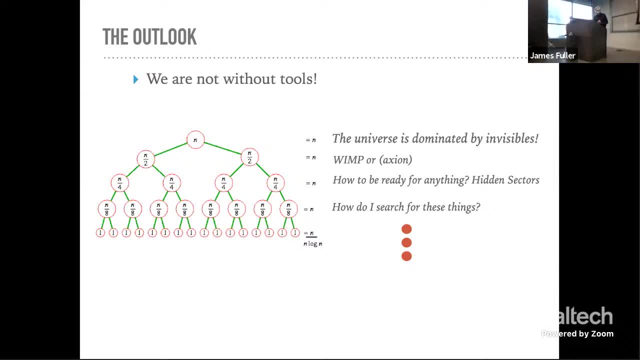 to catch up with the theorists, I think, the observers, experimentalists. Are there questions? First of all, if you're interested, I'm the audience here- You get the first dibs. Nancy, I need to be your friend. Thank you, Catherine. 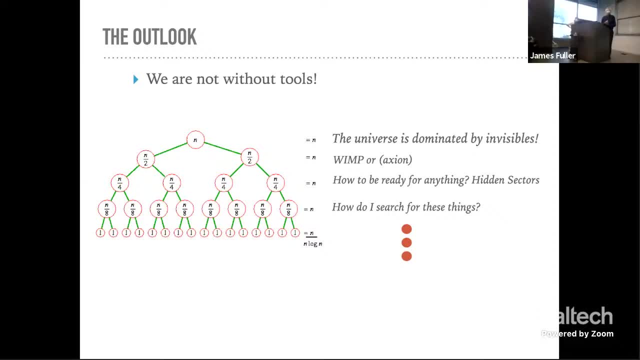 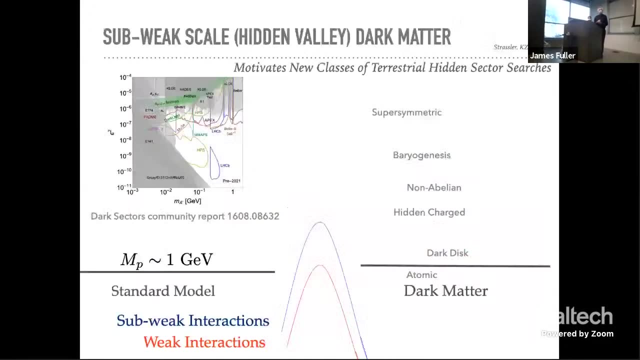 The question I asked you was about your class program that you can make an app cloud, where you mentioned that there's a disunity between the 12.5-year signal being at a specific level of this or dark matter-based transitions. So do you need more labs? 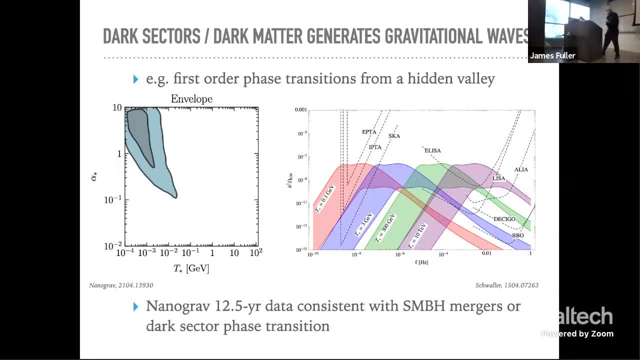 Are you small-scale More years? How do you? Yeah, So that's an interesting question. We have not done the study, So we worked with Nanograv to do this analysis, just to see if it was consistent. So in general, of course. 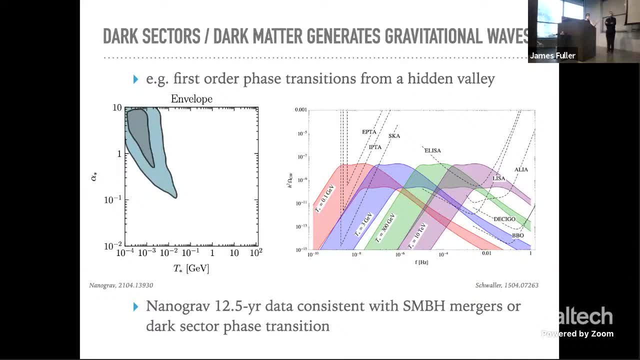 if you were able to make this measurement across a broad range of frequencies. the spectrum looks very different from a supermassive black hole scenario, because it's peaked with a frequency that's set by the phase transition temperature. So So, if you were just able to get a better handle. 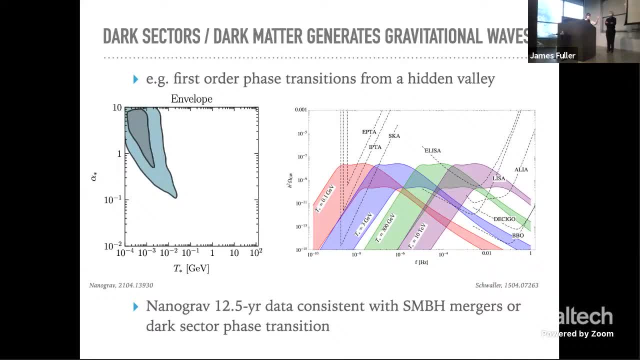 on the frequency spectrum over a broad range of frequencies in particular, that would already be because it rises and it falls, Whereas the SMBHB they're fitting just with a single power law. So the question is, how hard is that going to be to do? 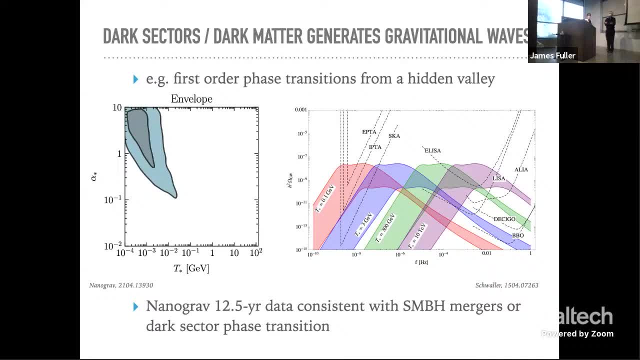 practically speaking, And I don't know the answer to that. But you know, I'm sure that there are experts in this audience who would have a much better idea than I would. George, I was intrigued by your model of non-electromagnetic. 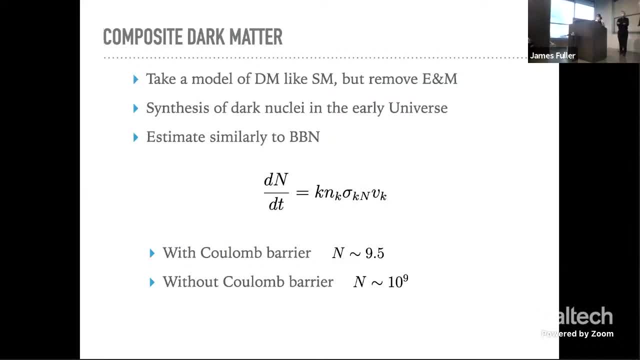 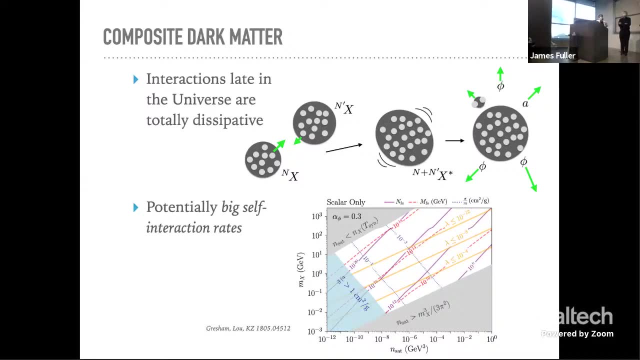 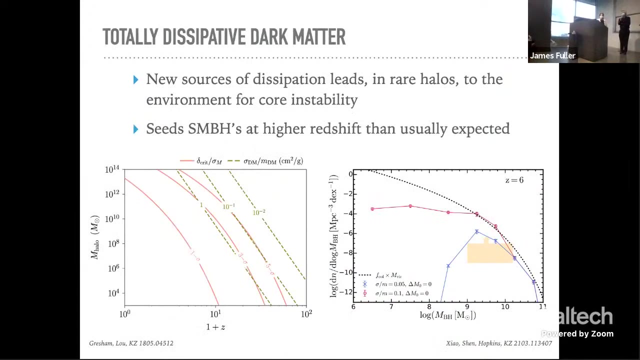 dissipation of things and creating these black holes? Yeah, Does that model also predict the correct radial shape as distributions for dark scales? Yep, On larger scales. So this is the. This is one of the keys. Can you repeat the question so that I can't hear you? 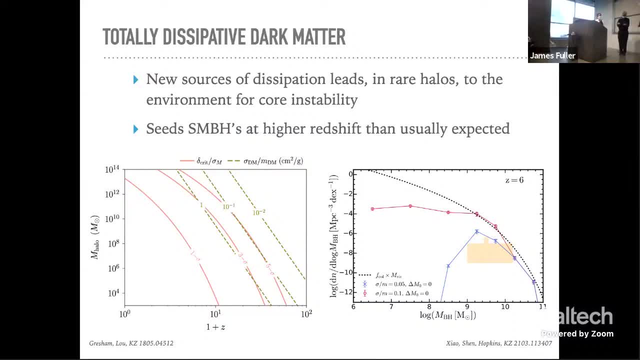 So he was asking whether, So if you can simultaneously see black holes and not actually create problems for the rest of what we know about dark matter, halos, If I can paraphrase your question that way. And the answer is yes, And we looked at that in quite a bit of detail. 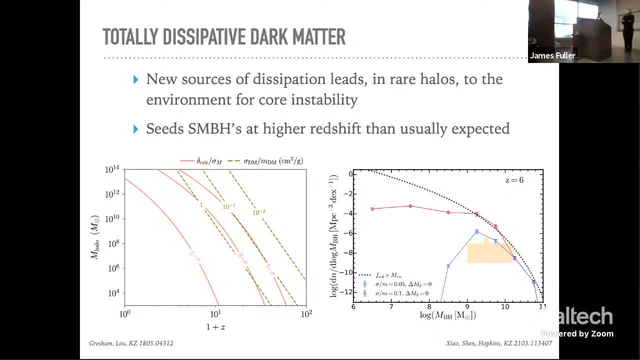 or I should say Jacob Huang Yu did. And the key here, or one of the key points, or one of the key ingredients here, is that you're looking at very rare halos, Okay, So most So the average halo does not experience this effect. 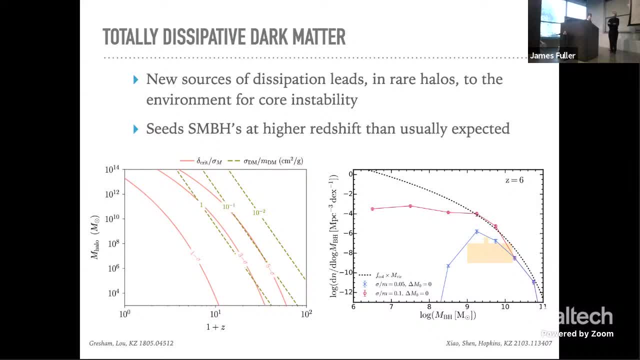 So you only need very, actually quite rare halos to have this occur, this instability occur, in order to explain what we see at high redshift. That's the short answer. So you know there'd be There's a much longer answer as well. 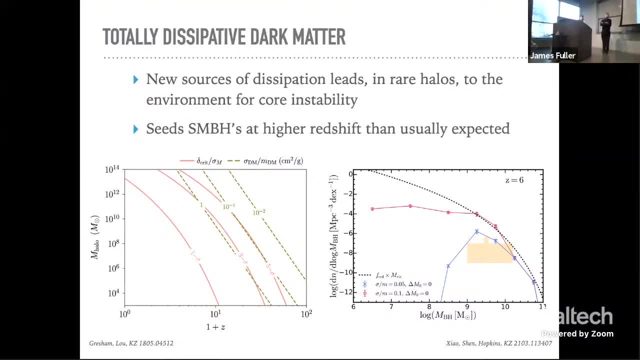 And I'm happy to talk about that later, Okay, Well, I mentioned the nature of the pulsar timing signal. Yeah, You mentioned it could be a background or perhaps an individual event that can dissolve. Yeah, But is there a chance or any likelihood? 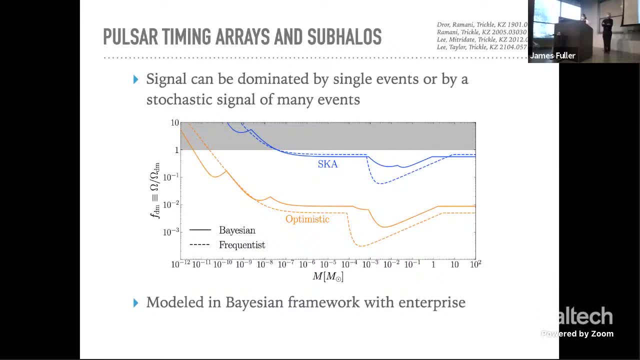 that it's correlated between pulsars, Because I think we've all now got a quite a heartbeat signal and we're not going to believe it until we see a correlation between pulsars. Yeah, that's right And, in general, the strongest constraints. 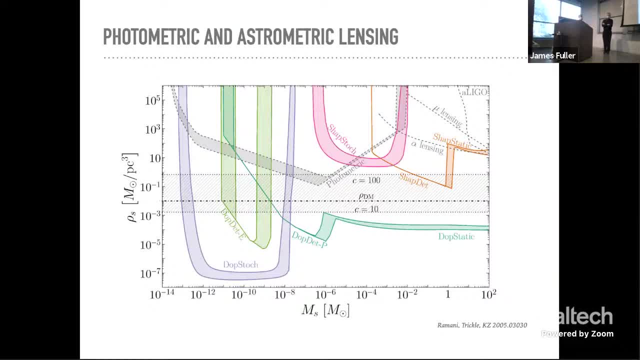 are actually coming from single events. So what we did? we did a variety of statistical tests, but the one that turned out to be the strongest, at least in certain parts of these. when we call something static or deterministic, what that means is that in that mass range, 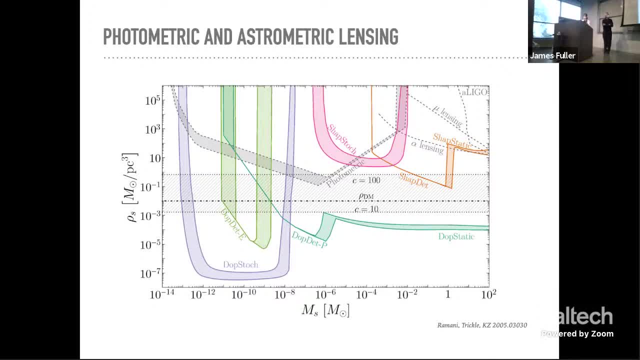 the most powerful constraint actually looked came from looking at a single pulsar with the single closest event that's coming by. That said, if, for example, you can see that this Doppler signal here actually dominates over this whole range, that means I'm pulling on the pulsar. 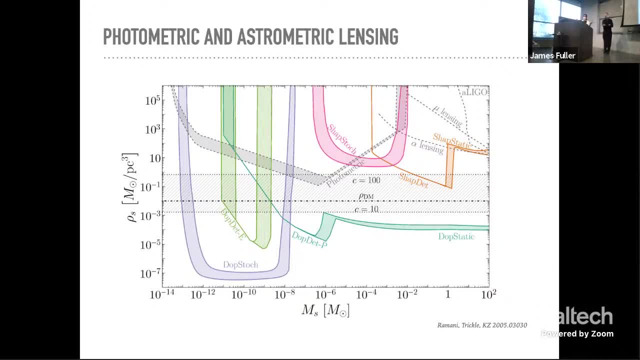 and that's a dipole. Okay, so that's very specific. So you should be able to see that And if I have a hope that you'd be able to separate this from a, you know, a stochastic background, If that whole segment. 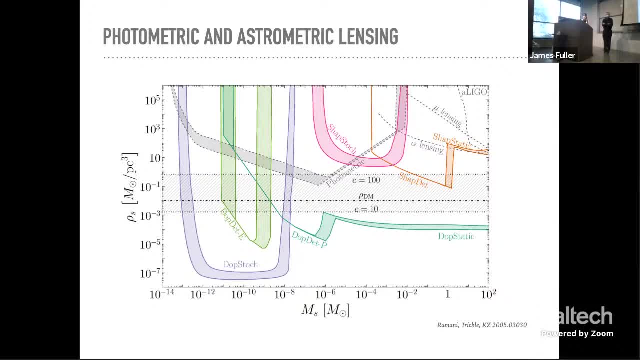 that whole segment holds now going forward it's going to be the combination of a different frequency. dependence, because this is actually this- accumulates, So it doesn't just depend on T minus T prime, it also depends on T, And so that's also different from a stochastic background. 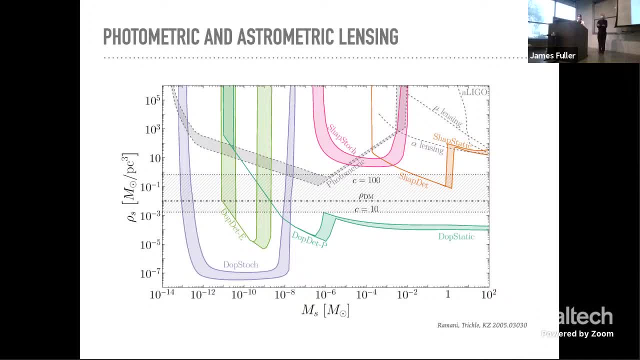 So there are a few different handles that, if one really dug into it, I hope that one could use those to try to distinguish this type of a signal from the stochastic background. But it is not something that we've dug into yet in detail, Shree. 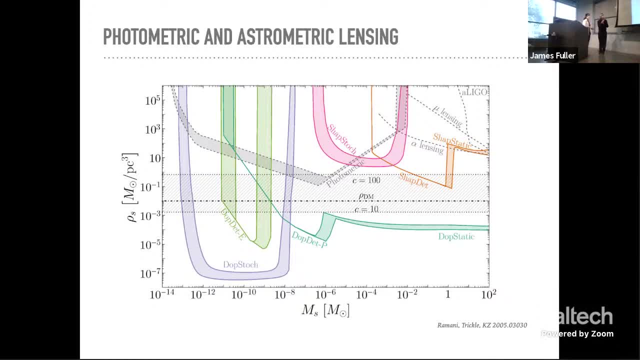 Yeah, I'll just dive in. There's another method you can have applicable around roughly one solar mass in a decade around it, which is faster than most. It's distinctly different from all the other techniques. Basically the It's sort of it's lensing, but now you get the rays that are lensed in the field. 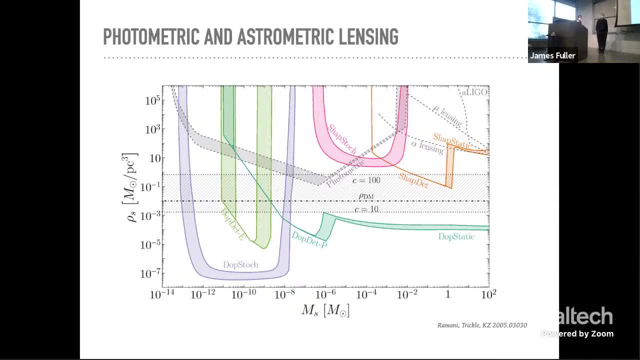 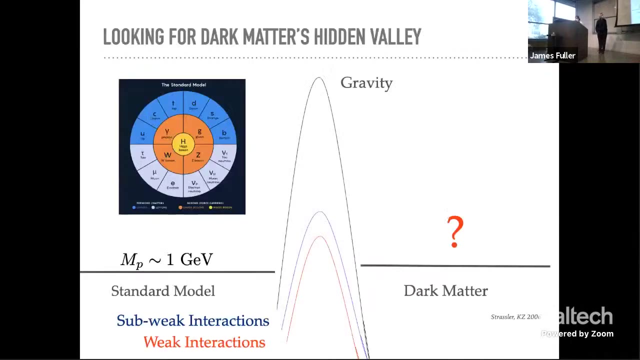 in the ordinary magnetic sense and you get the fringes that you see the faster because I think I don't know where I think those signals would be very, very So I think it might have actually been on my black hole plot. 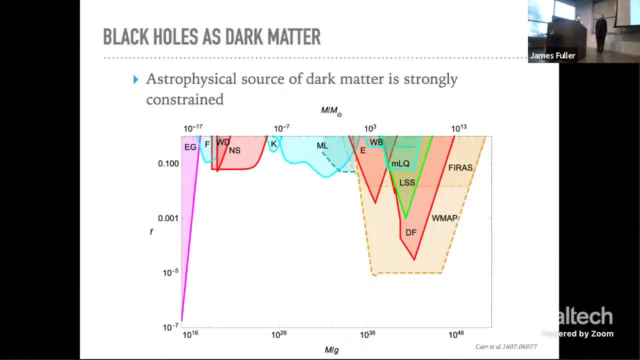 17. So you're saying that fast radio bursts, basically lensing of it, you can get a fringe pattern from a dark matter. you know, usually people are looking at this in the context of astrophysical black holes that would be passing between the fast radio bursts and us. 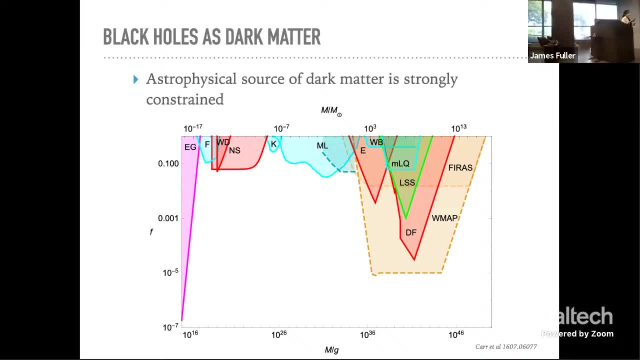 Yeah, it doesn't have to be a black hole. That's a good concentration. Yeah, and I thought that actually came in at much lower mass. It's not at a solar mass. I thought that was actually further down here somewhere. I thought that was what this F was- at much lower mass. The other comment I want to make about that: 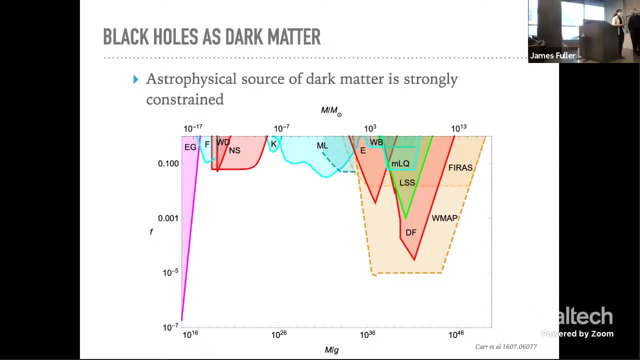 though is, I can look up the exact numbers, but I think that that constraint actually, and many of the lensing constraints also require that the halo be extremely dense, like extremely dense. So even these like axion mini clusters, which are already quite dense, 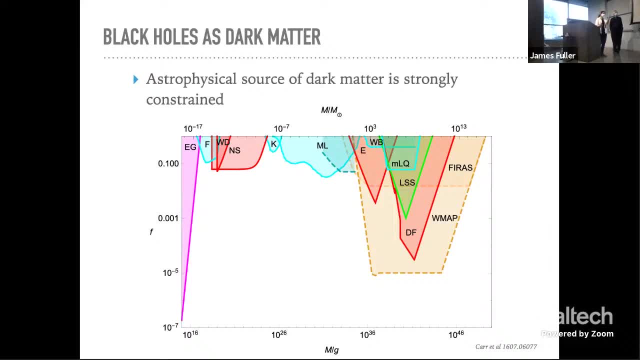 it just wouldn't be able to see them because they're too fluffy, because it's such a small angular resolution measurement, And so that is the other part of it. that I tried to emphasize is that, you know, lensing is very, very powerful for extremely. 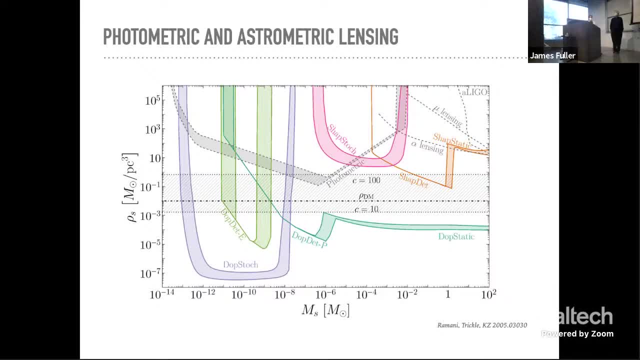 dense objects, So it works well for machos, but in fact across this whole mass range. But they don't apply at all to these objects because they're just too fluffy, Like even things that are much, much more dense than CDNs. 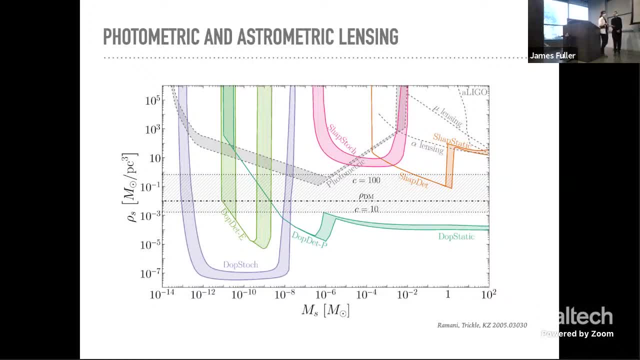 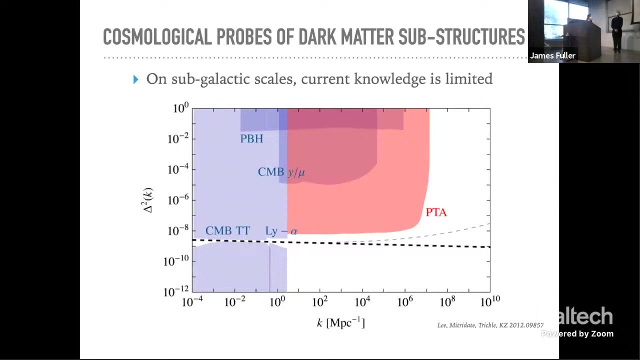 halos you can't see with lensing, because the concentration just isn't high enough. Yeah, go ahead. So I think this is probably what you're talking about. Oh, yeah, So the question was whether CMB spectral distortions can be a probe. 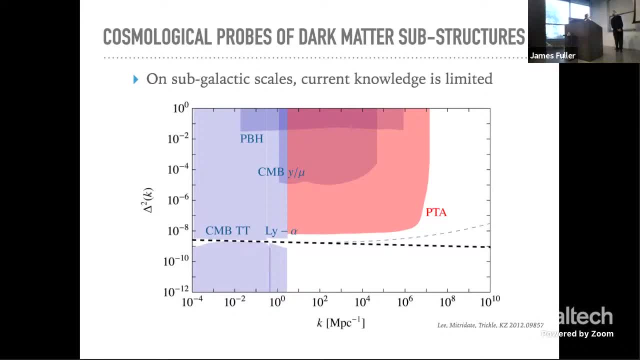 And the answer to that is absolutely yes, And that's what's shown here. Yeah, I don't know exactly where they are, But yes, in this kind of range. So they would be sensitive to larger density perturbation. So, again, that's going to correspond to: 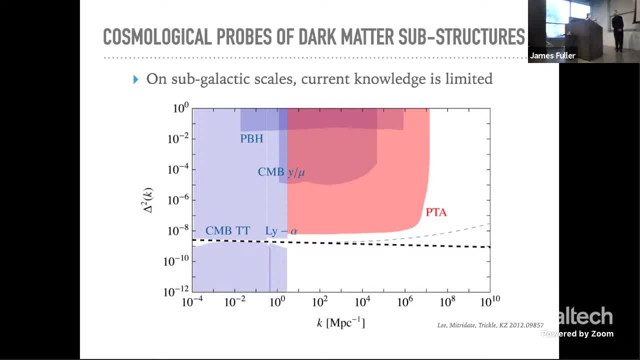 very high, very high concentration. And so you know, in terms of models, theories of dark matter, that would create halos that would be dense enough. even many clusters are very dense, But they're still not dense enough to be seen. Well, there are much smaller mass scales. 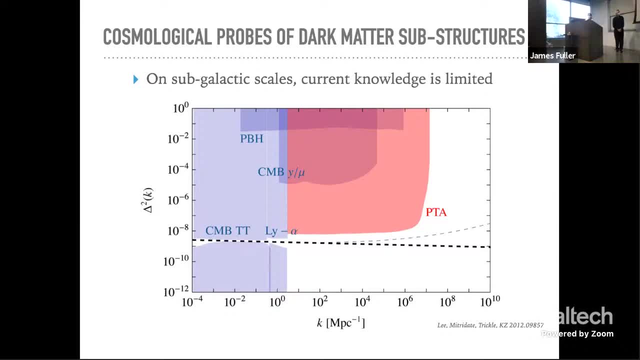 But there are some theories that that would probe is the short answer here: Questions. Any more questions in the room? Are there any questions online? Yeah, there's one online, Okay, Okay, Can you repeat the question? a halo, mass, black hole, mass relation, um. 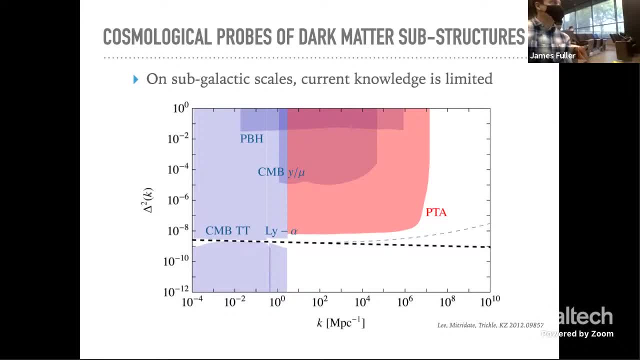 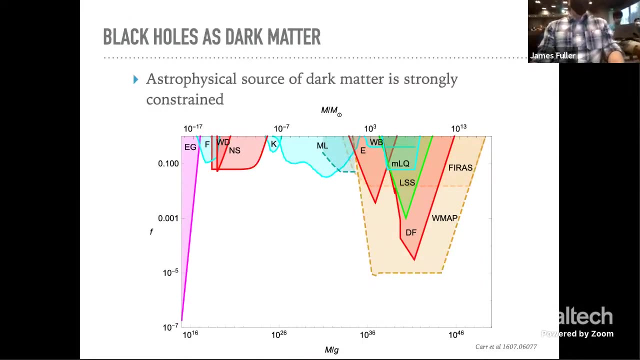 not that i'm aware, but i- uh, i- have not studied primordial black hole formation, and the primary reason for that is that, when you look at it from an observational point of view, what you're trying to do is dodge this, so you can dodge this, and, in fact, in fact, people do try to.